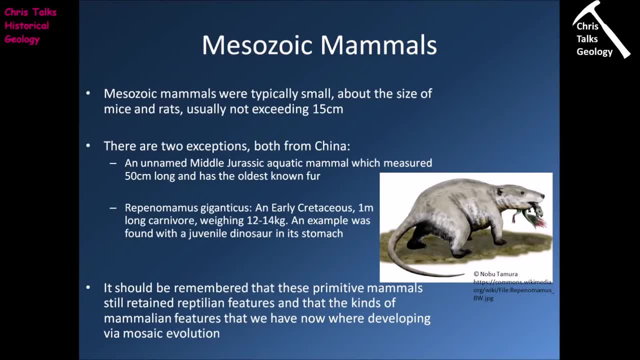 reach this large size is very likely because it's operating in the aquatic environment, And this means competition with other groups of animals like the dinosaurs and reptiles in general would probably have been lower, And this would have allowed it to have, you know, become a major. 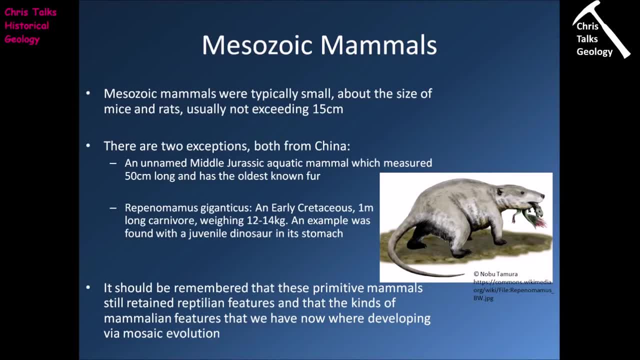 predator within this particular environment, So that would have helped it to allow it to reach its larger size. Now the other organism is an organism called Repenemamus, And this is an early Cretaceous one meter long carnivore that weighed about 12 to 14 kilograms. So this is a little bit. 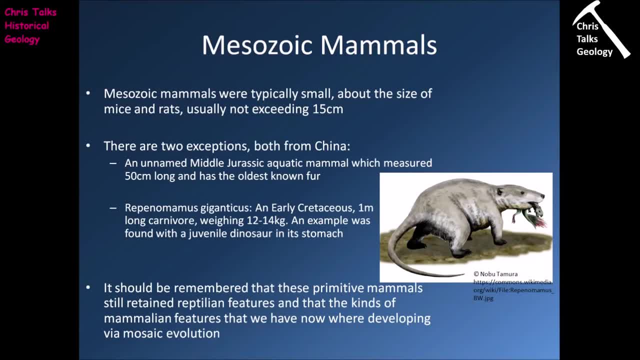 bigger than a Cretaceous one meter long carnivore, So this is a very sizable animal. Now, this one is of interest to us because one of the fossils that we found of this particular organism has its stomach contents fossilized And as part of that stomach contents, 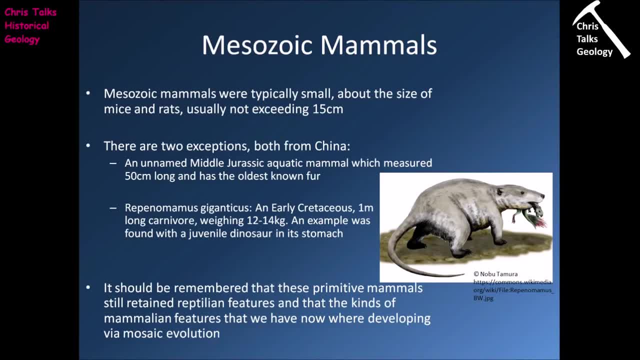 we can see that it contains the bones of at least one juvenile dinosaur. So it should be remembered that these primitive mammals still retained reptilian features and that the kinds of mammalian features that we're used to now, like the free-boned inner ear, the differentiated teeth, 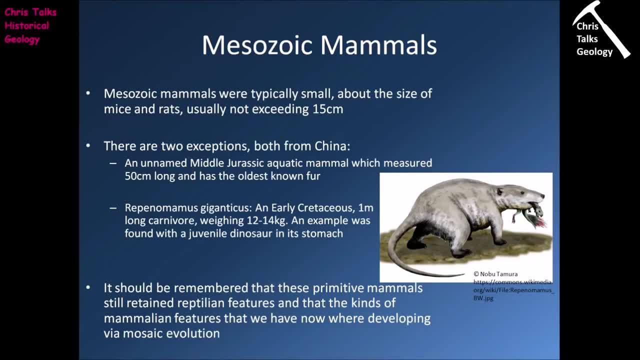 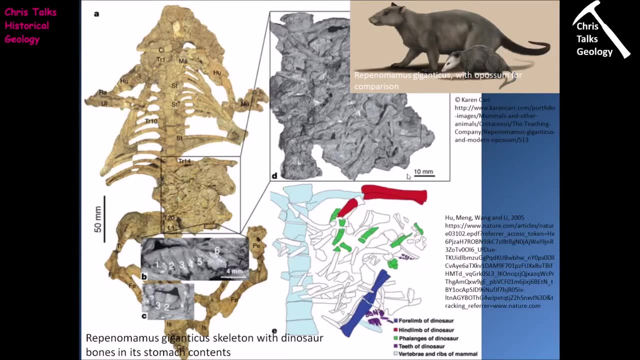 etc. were in the process of developing via mosaic evolution, And so this means that, yes, these organisms would have looked like mammals to us, but there would also have been subtle traits which would have hinted at their reptilian lineage. So here we actually have the fossil of the 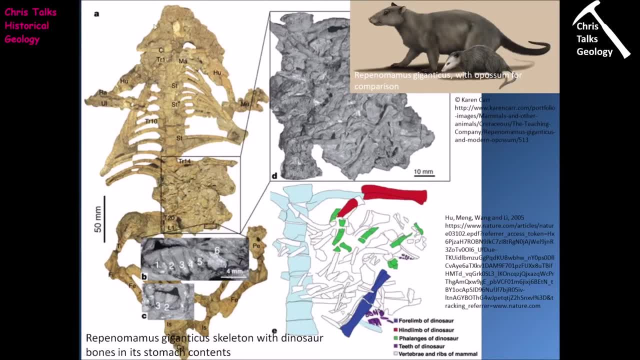 Repenemamus organism in question. So we can see the head would have been located up here at the top and the tail would have been down at the bottom. We can see the spinal column coming straight down there. We can see the head would have been located up here at the top and the tail would have been down at the bottom. 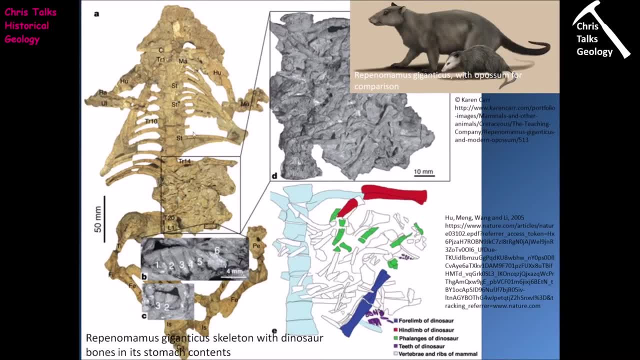 So we can see. the head would have been located up here at the top, and the tail would have been down at the bottom. One forelimb here, another forelimb here. obviously, the rib cage is there, pelvis is down here. 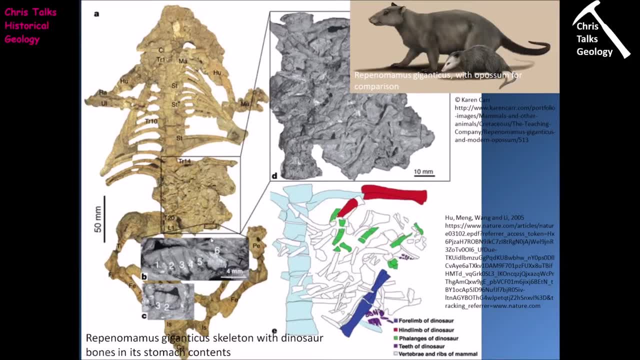 And right here you can see a collection of smaller bones and bone fragments And this is actually the picture of it blown up And this is a map of the bones in this area. So we can obviously see we have the spinal column of the Repenemamus right there. 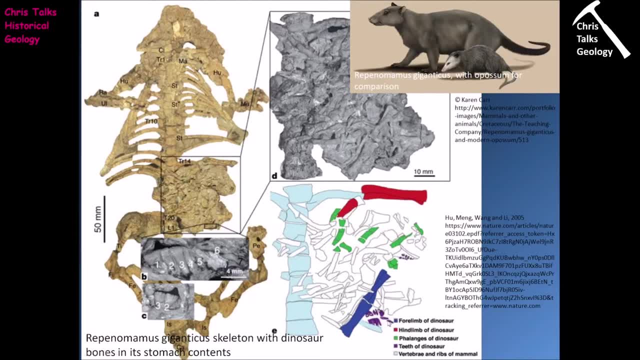 And then we have this collection of bones right here, and as part of this collection of bones we can see we have the hind limb of a dinosaur here, here in red, the phalanges of a dinosaur in green. remember, phalanges are finger and toe bones. 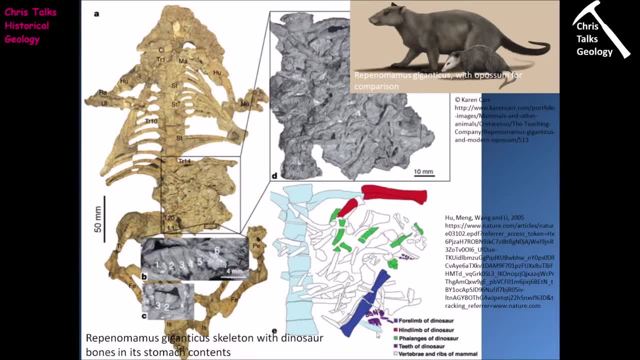 the folium of a dinosaur in blue and the teeth of a dinosaur in purple, and these bones show indications of having been essentially chewed, so we can see teeth marks in them and we can even see some indications of acid damage, and so this is showing us that you know, this is clearly a prey. 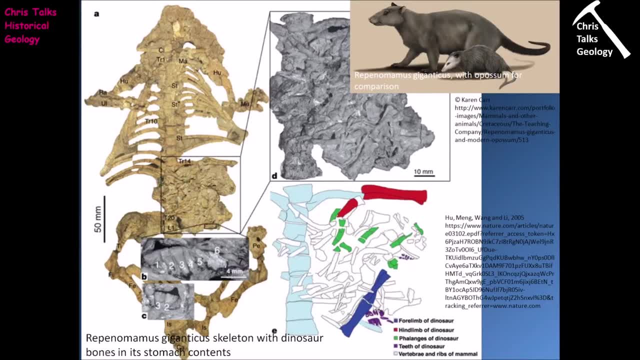 item that's, you know, in the stomach. so this is showing us that you know. this particular large mammal was an active hunter and as part of its diet it went after small dinosaurs. and just to give you some idea of the size of repinomamus, here's a picture of it compared to a modern day. 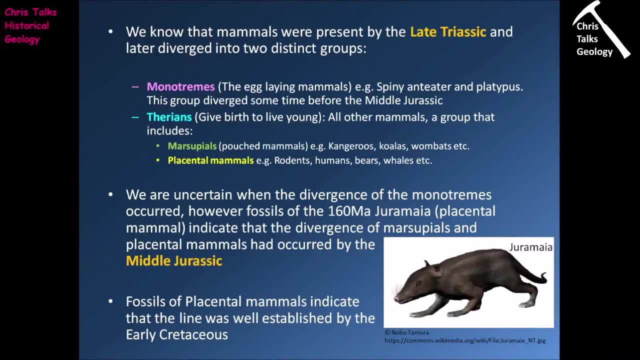 possum. so when we look at the fossil record, we can see that mammals were present in the mesozoic by the late triassic, and these mammals would later diverge into two distinct groups. so the first group are the monotremes, so these are the egg-laying mammals and this is a 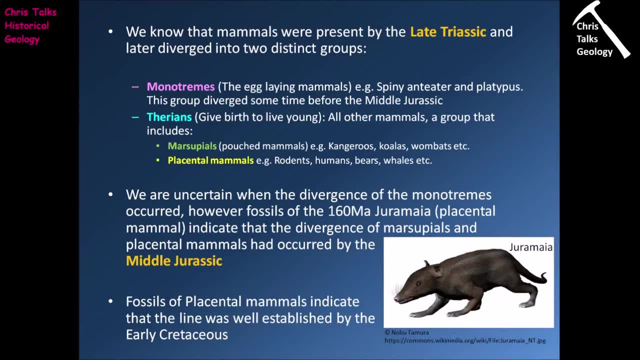 group that includes the spiny anteater and the platypus. now, in terms of the divergence of this group from the main mammalian line, it looks like it probably happened sometime before the middle jurassic. we're not 100 sure when. now the other group are the therians, and this is a group of 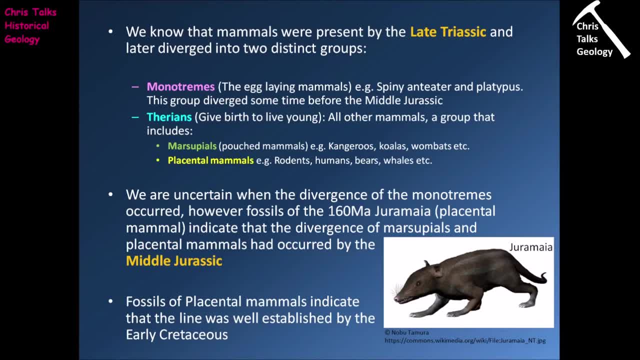 mammals which give birth to live young. so essentially this is every other mammal with the exception of the monotremes. so this group contains two important subgroups: the marsupials and the placental mammals. so the marsupials are the pouched mammals, so that's organisms that include kangaroos, koalas and 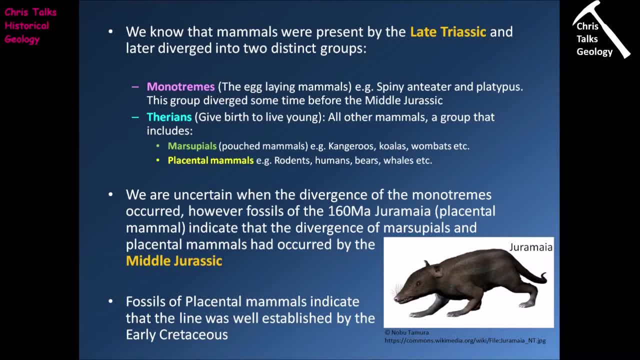 wombats and the placental mammals is a group essentially that contains the other remaining mammals, so that's groups like the rodents, the humans, the bears, the whales, the cats, the dogs, etc. now, as i said, we're uncertain when the monotremes diverge from the spiny anteater. 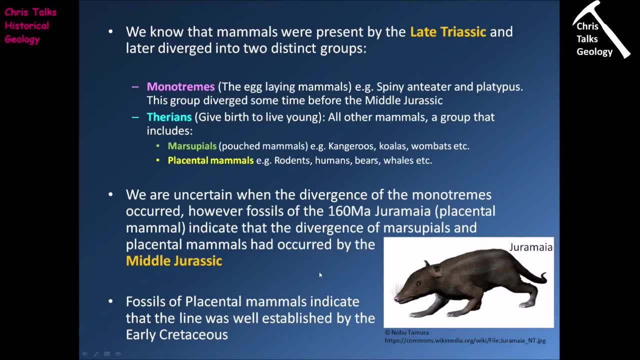 line. however, we do have some general timing evidence for this divergence in the form of a 160 million year old fossil from china called jeremiah. now, jeremiah is a placental mammal, and so this would indicate the divergence of the marsupials and the placental mammals. 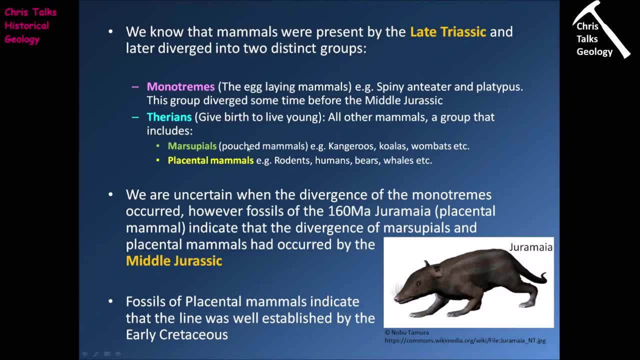 sometime around the middle jurassic. now this obviously means the monotremes must therefore have diverged from the mammalian line but not from the spiny anteater line. so this is a group before the middle jurassic, because of course the placental mammals are part of the therian group. so 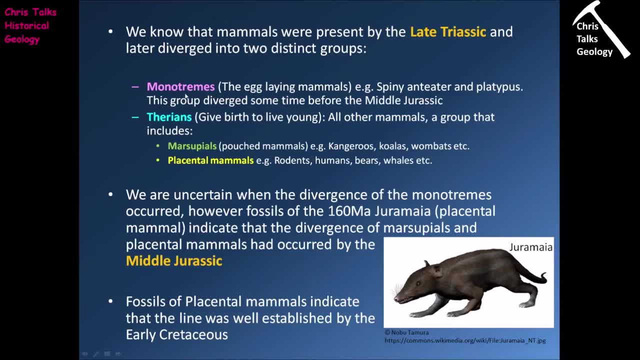 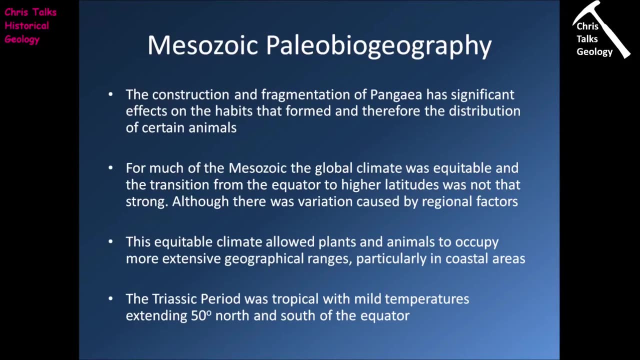 we know, in order for the therian group to have existed, the monotremes must have branched off earlier. now, fossils of placental mammals indicate that the line was well established by the early cretaceous. so now we're going to spend some time thinking about how the breakup of pangaea and the 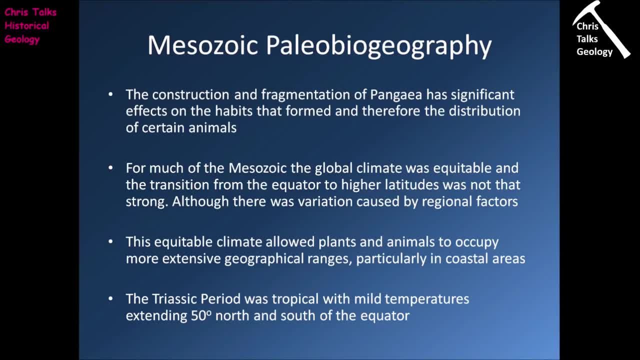 movement of the continents towards their current position ended up affecting life in the mesozoic. so we are going to spend some time looking at mesozoic paleo biogeography, which is quite the mouthful. so the construction and fragmentation of pangaea has significant effects on the habitats. 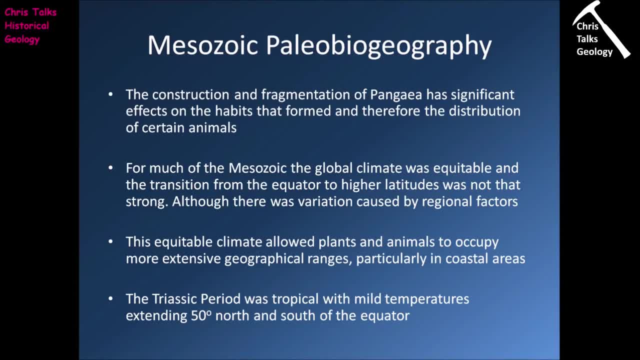 that formed, and therefore the distribution of certain animals, as you would expect. so for much of the mesozoic the global climate was, on the whole quite equitable, and the transition from the equator to the higher latitudes was not that strong, so warm conditions continued towards the poles for quite a long way, and so this would have made the environment quite nice, and 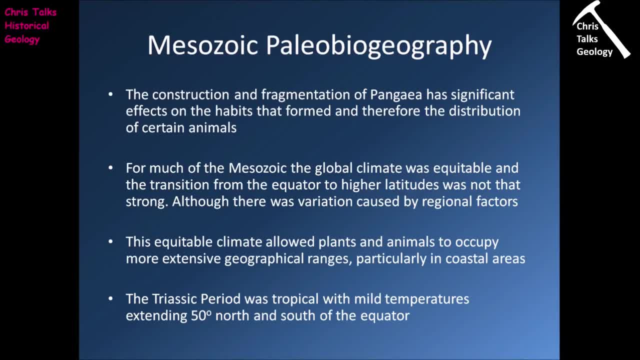 quite you know, hospitable to most organisms. now, there would have been some local variation caused by regional factors such as mountain ranges, but on the whole conditions would have been quite nice. now this rather you know nice- climate allowed plants and animals to occupy more extensive geographical ranges, particularly in coastal areas where there was lots of water available. 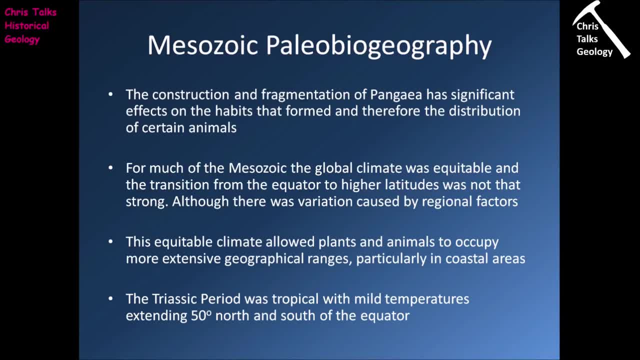 and so what? you have a situation where you have nice conditions. obviously that's going to help plants to be able to grow pretty much anywhere, and as long as the conditions are met, such as a reasonable amount of water, the plants will inhabit that area and they will typically prosper. so the triassic period. 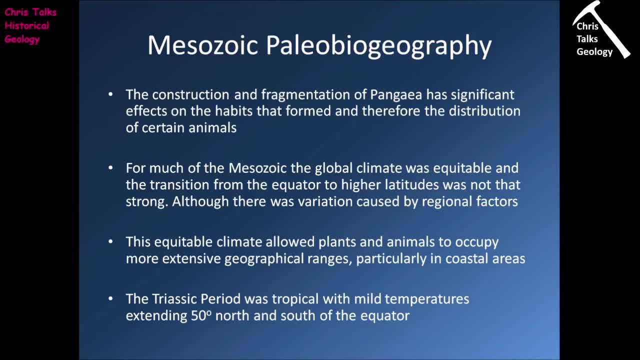 was on the whole tropical, with mild temperatures extending 50 degrees north and south of the equator. so this means you know you have a very, very broad warm band around the midpoint of the earth that extends 50 degrees from that grid, so that's a very large area of the earth surface. 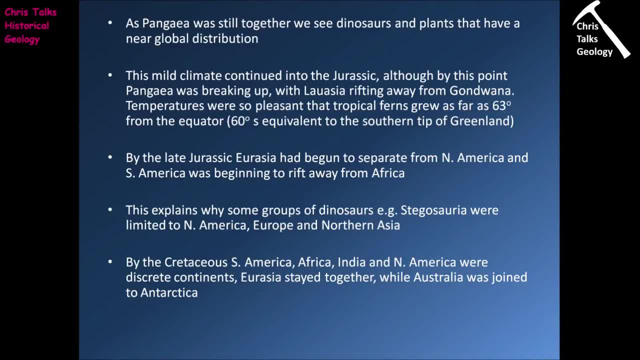 where conditions would have been quite nice now, as pangea was still together in the trassic, we see that dinosaurs and plants from this period have a near global distribution and of course this makes quite a lot of sense because the continents are all joined together. it would have been relatively 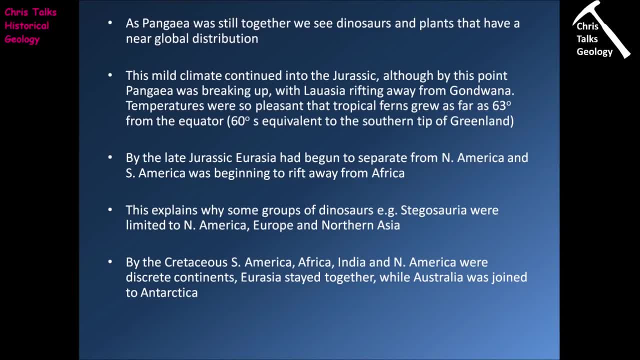 easy for animals to have migrated from one landmass to another. now, as we move from the triassic into the triassic, we see that the mild climate continues, although, of course, by this point pangea has broken up into two large land masses. we have laurasia in the northern hemisphere, so 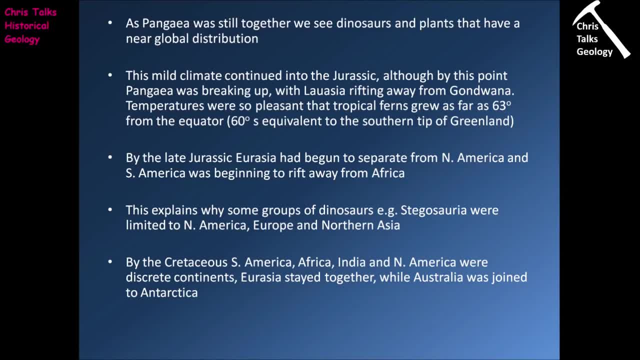 that's north america, europe and asia, and we have gondwana in the southern hemisphere, that's south america, africa, india, australia and antarctica. now, in terms of the uh nice, uh climatic band which we saw in the trassic, this nice band persists into the jurassic and it actually 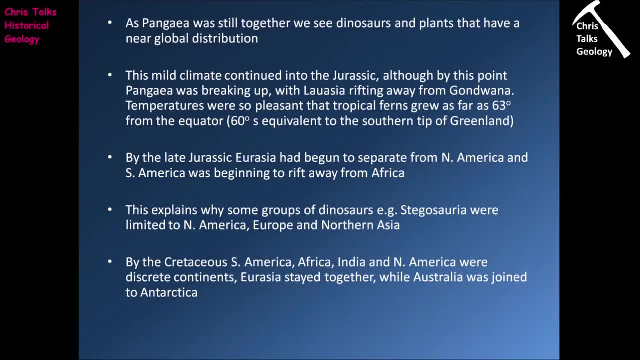 gets a little bit wider, and so in the jurassic we can see that we have tropical ferns growing as far north as 63 degrees from the equator. just to give you some idea, 60 degrees north of the equator is equivalent to the southern tip of greenland, and so this means that during the 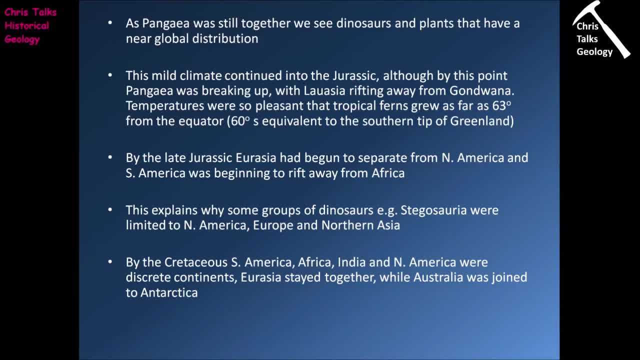 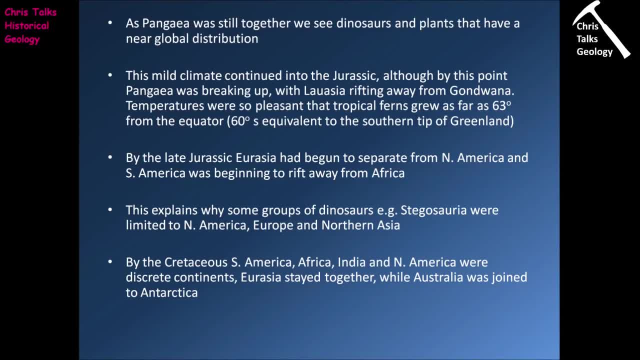 very, very good. obviously you had nice warm weather, as long as you had enough rain water and good enough soil. this obviously would have allowed plant life to flourish, and so that would mean there would be plenty of food for large herbivores, especially the dinosaurs. Now, by the late Jurassic. 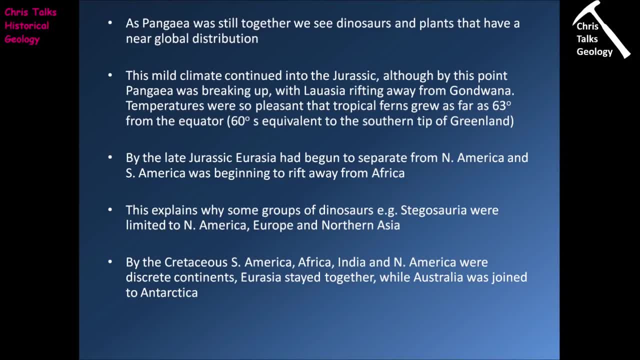 we see that Eurasia and North America are beginning to separate Now. to be clear, the separation of North America and Eurasia takes a very long time and we don't see the two land masses actually fully separating from one another until the very, very end of the Cretaceous. So what I'm saying. 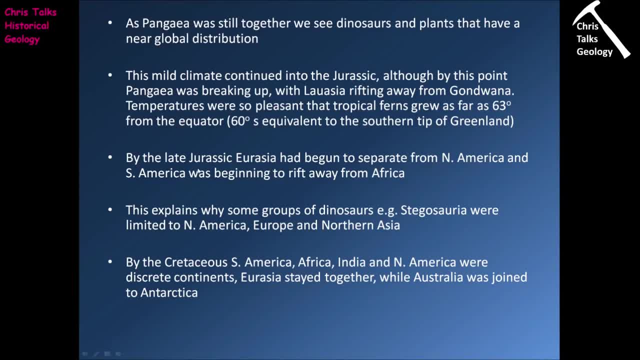 here is. we see the first signs of North America beginning to rift away from Eurasia in the Jurassic, but we don't actually see the two land masses become independent from each other until the end of the Cretaceous. So this means that during the Jurassic and for much of the Cretaceous, 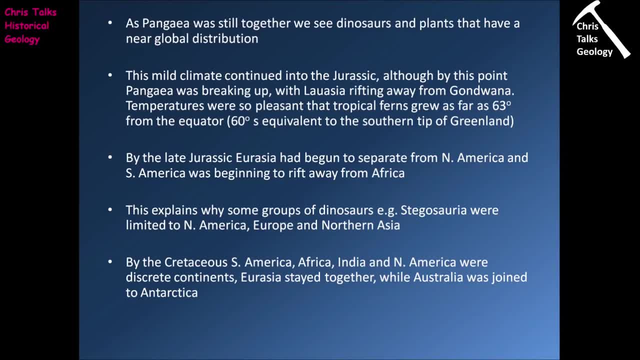 it would have been possible for animals to separate. In terms of what's going on down in the southern hemisphere, we obviously have the breakup of Gondwana, so we have South America and Africa rift off, another land mass which is made from India, Australia and Antarctica, and then by the middle Jurassic. we begin to see the first stages of South 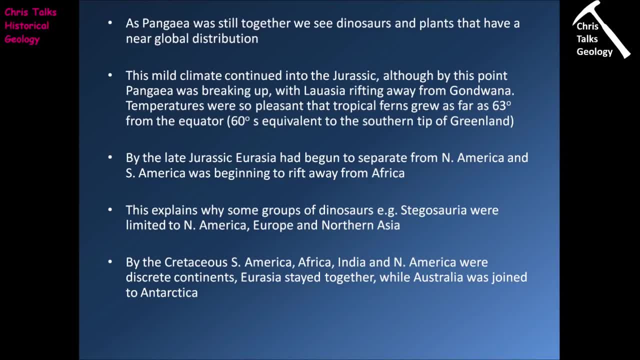 America rifting away from Africa. Now the breakup of Pangaea begins to explain some of the factors which we see in the distribution of certain groups of dinosaurs. So a good example are the Stegosaurian dinosaurs. So we see that they are exclusively limited to North America. 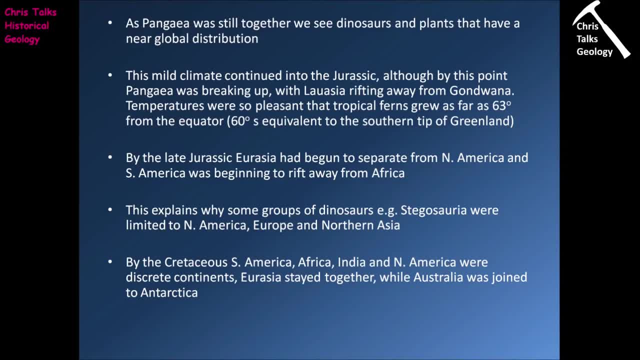 Europe and Asia. and of course this makes sense because during the, during the Jurassic, North America, Europe and Asia formed one large land mass, so the Stegosaurs could have obviously migrated across, you know, with relatively little fuss. In contrast, the southern hemisphere continents were completely separated from the Stegosaurian dinosaurs, So we see that they are exclusively 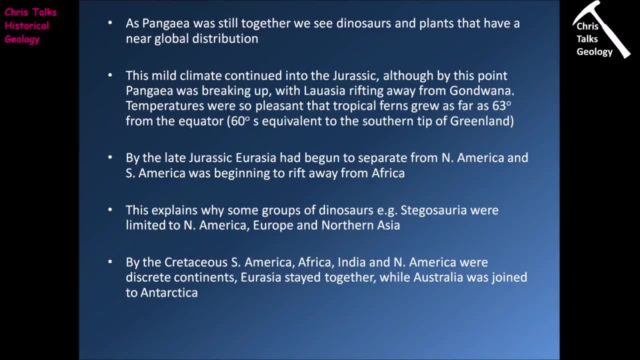 limited to the southern hemisphere continents by a large body of water, and so this would have therefore made it impossible for the Stegosaurs to have ever made it onto the southern hemisphere continents. so they're just not present in the fossil record of those land masses. So by the 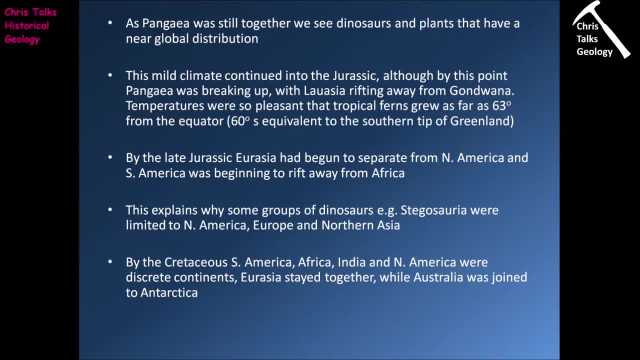 Cretaceous. we see that South America, Africa, India and North America are operating as discrete continents, although Europe and Asia stay together as one land mass and Australia is still joined to Antarctica for a very large portion of the land mass. So we see that South America, Africa, India, 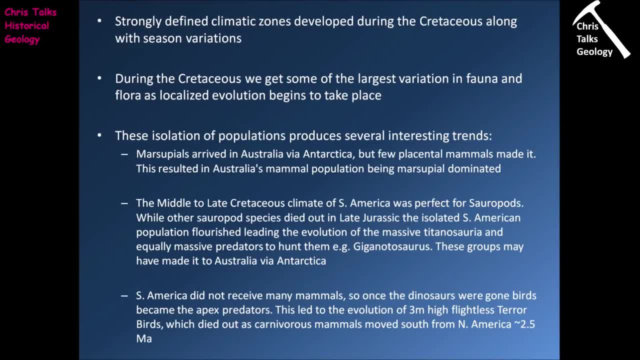 are operating as discrete continents, although Europe and Asia stay together as one land mass. So we see that Cretaceous are operating as discrete continents, although Europe and Asia stay together as one land mass. So, because the climate, because the continents are moving towards their current positions, we begin. 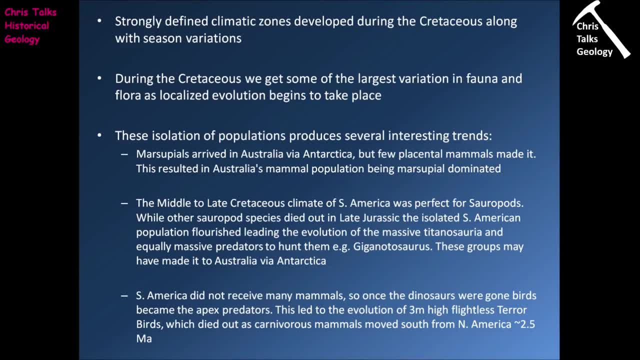 to see strongly defined climatic zones beginning to develop and within those climatic zones we also see the formation of seasonal variation. So we've already discussed that the movement of the continents is going to affect the circulation of water in the oceans and air in the atmosphere. 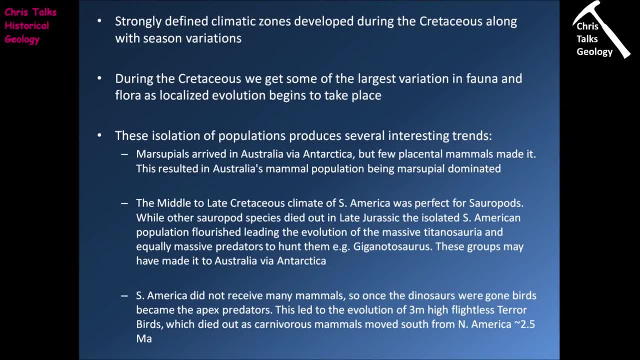 and this is obviously going to have an effect on climate. We've also discussed how the movement of continental crust northwards and southwards, towards the north and south pole, essentially replaces seawater, which is present, which was present, should I say, at the poles in quite large quantities during the Triassic and Jurassic. 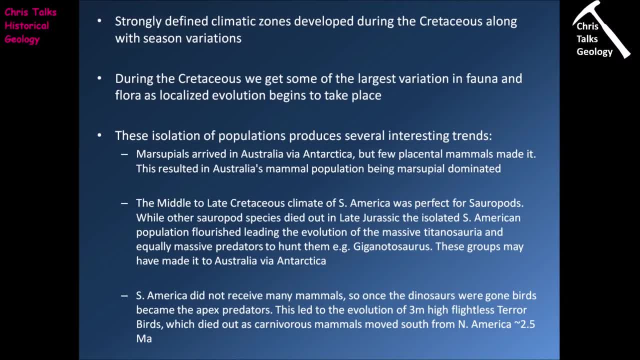 with continental crust. The problem is that seawater is very, very effective at absorbing and retaining solar radiation, so it helps to keep the area warm. In contrast, continental crust is far worse at absorbing and retaining solar radiation, so it doesn't retain as much heat. and so this means, as Antarctica moves towards the south pole and as North America, Europe and Asia. 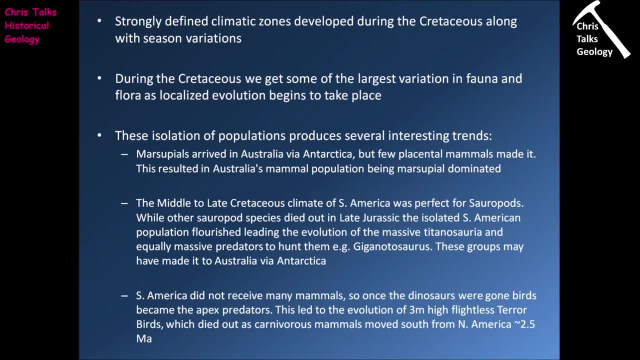 move towards the north pole, we are essentially replacing seawater, which is very good at absorbing heat, with continental crust, which is pretty rubbish at absorbing continental heat, solar heat, and so this means that we begin to see a temperature decrease in the polar regions. So as we move into the Cretaceous, things are getting a little bit more variable, shall we say. 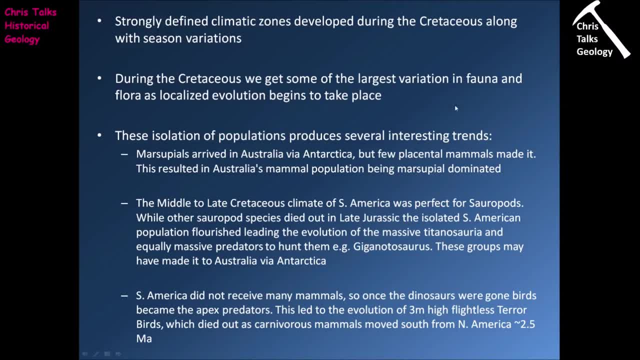 Now, during the Cretaceous, we get to see some of the largest variation in fauna and flora during the Mesozoic, and this is because we are setting up these localized environments in which evolution will have to specialize the animals. So these isolated populations for each of these different continents produce several interesting 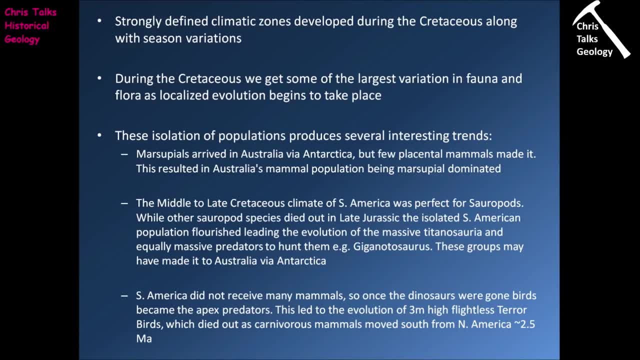 trends. So, in the case of Australia, we see that the marsupials arrive in Australia via Antarctica, but very few placental mammals make it to Australia, and so this means that, in terms of the makeup in with regard to mammals of Australia, we see that it's dominated by the 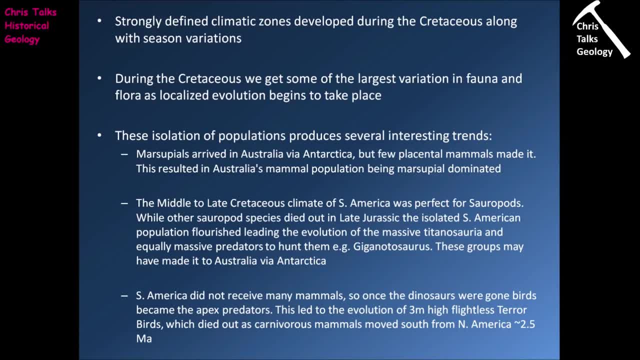 marsupials and placental mammals are a relatively minor component. Now, this actually also held true for South America. For a very long period of time, South America's mammal population was also dominated by the marsupials. however, what we saw is we saw the marsupial population population being hit quite hard. 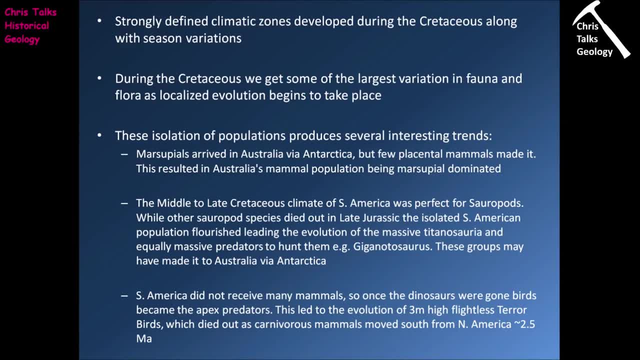 when North and South America joined together, because this then allows the placental mammals of North America to move south and they begin to out-compete the marsupials of South America pretty effectively. So we also see that the middle and late Cretaceous climate of South America was perfect for the sauropods. 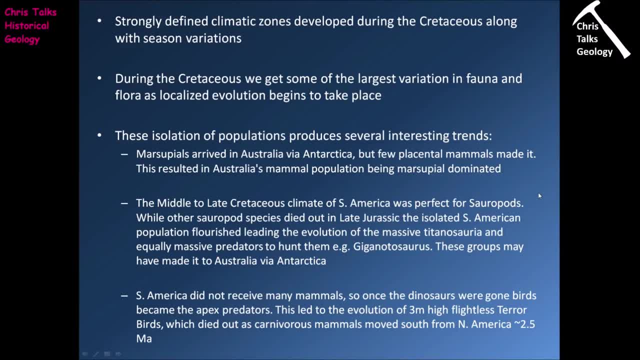 So when we're talking about the rest of the world during the Cretaceous- so North America, Europe, Africa, etc. conditions are getting quite hard for the sauropods, and so we begin to see sauropod populations dropping off and we begin to see numerous sauropod species becoming extinct. Now this doesn't happen in South America. 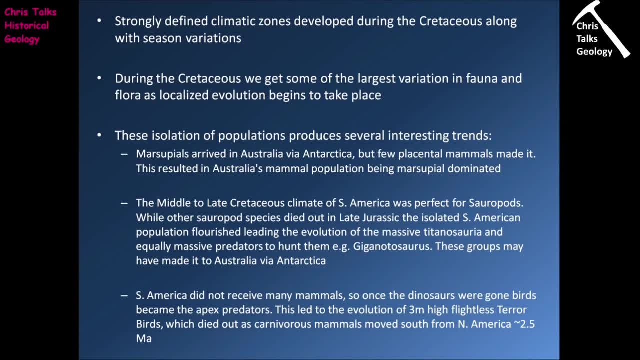 because conditions are actually quite high, absolutely perfect for the sauropods. and so what we see in south america during the cretaceous is we see the evolution of the largest of the sauropods, the titanosauriforms, and so these titanosauriforms is absolutely huge herbivores, of course, get preyed on by predators, and so, as the 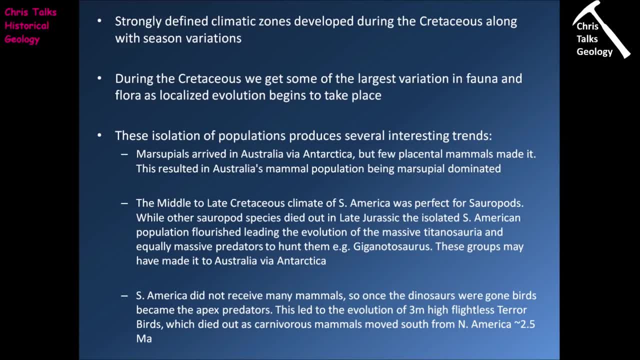 herbivores get larger, so must the predators, and so we also see in south america, during the cretaceous, we see the evolution of absolutely massive carnivorous dinosaurs, so that's organisms like gigantosaurus, because there's this arms race between the titanosauriforms and these very, very 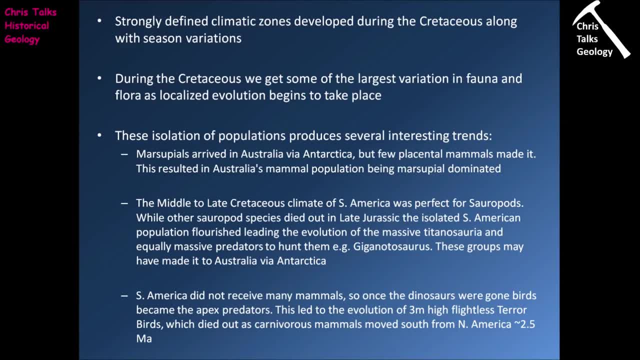 large predators. now, in terms of titanosauriforms, there's some evidence to suggest that some of them might have actually made it all the way to australia, so that would have meant they would have had to have migrated from south america to australia via antarctica, and of course that's. 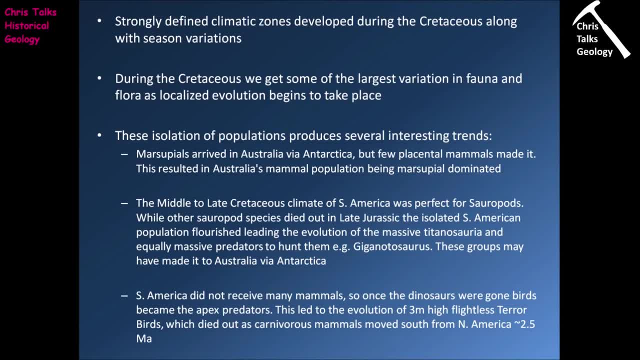 possible because for a relatively long period, south america, antarctica and australia would have been joined together as one landmass. now, south america did not receive many mammals. so once the dinosaurs were gone- so we're talking, you know, in the early cenozoic we actually see the 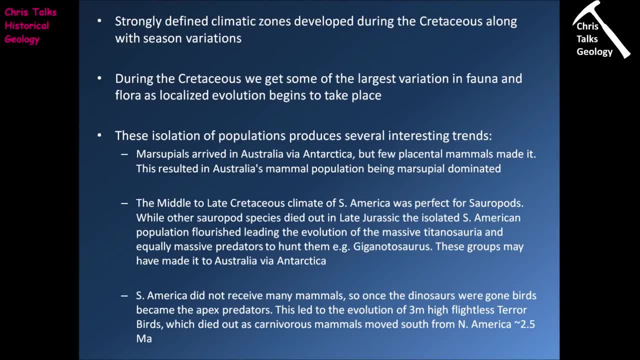 birds becoming the apex predators in south america, and this actually leads to the evolution of the three meter high flightless terror birds, as they're called, and, And these birds did very, very well once again, until North and South America become one large landmass. 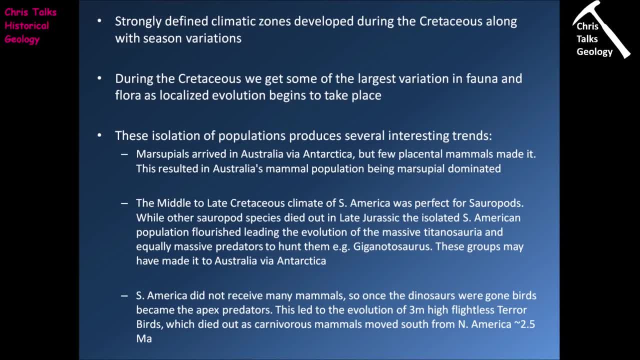 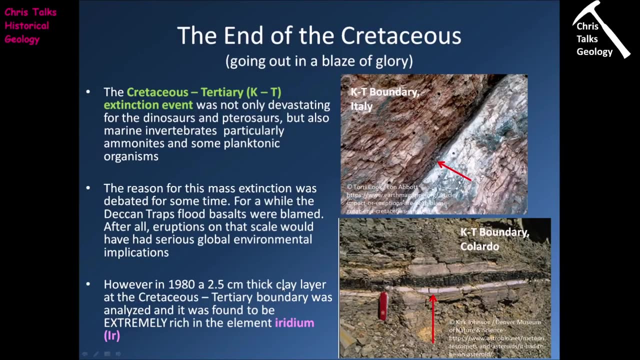 At that point, placental mammals from North America migrate southwards and they end up out-competing the flightless birds quite quickly. Now we'll actually cover this process as part of the Cenozoic Life History Lecture. So let's talk about the end of the Cretaceous and also, obviously, that means the end of the dinosaurs. 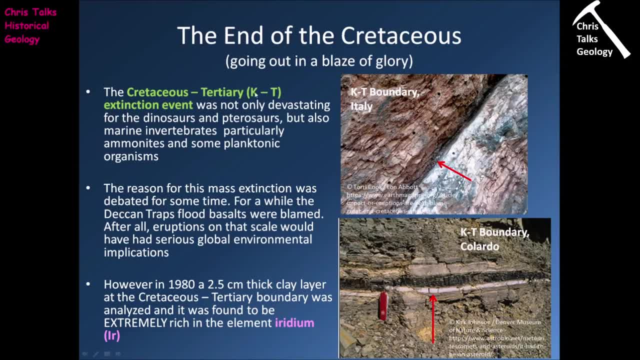 So the Cretaceous-Tertiary boundary, which is sometimes referred to as the K-T boundary, marks an extinction event. Now, this extinction event was not only devastating for the dinosaurs and the pterosaurs, but it also did some pretty serious damage to marine invertebrate communities. 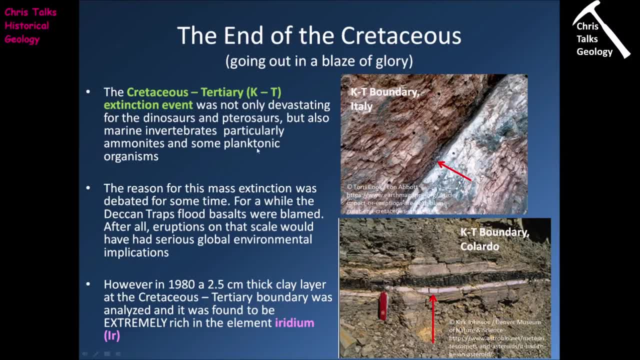 So we see the ammonites and we see the rudists and we see lots of different types of plankton. So we see the ammonites and we see the rudists and we see lots of different types of plankton. 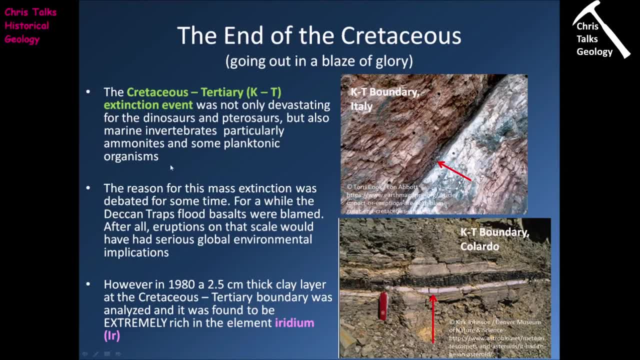 So single-celled photosynthesizing organisms dying out at the end of the Cretaceous. Now, the reason for this mass extinction was debated for some time. For a while we thought the Cretaceous-Tertiary mass extinction was due to the Deccan Traps, flood basalt eruptions which were taking place in what is now modern-day India. 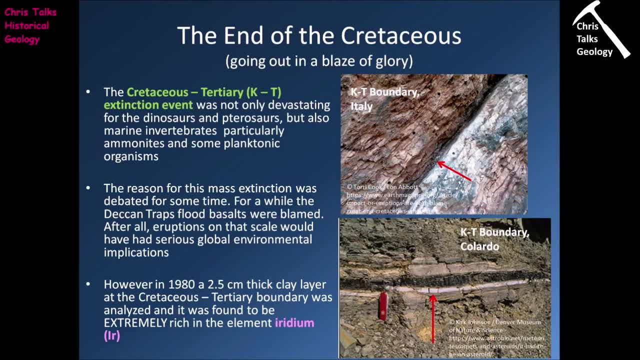 So in that area during the Cretaceous, we have huge fissure eruptions pouring out vast quantities of magma onto the surface of the Earth, And the model went that the carbon dioxide that was being pumped into the atmosphere ended up causing a greenhouse effect. 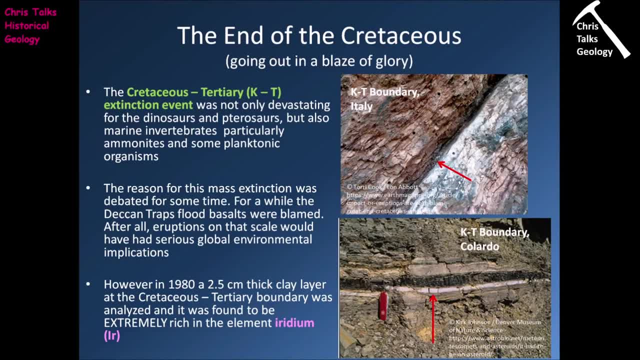 Combine that with all the other gases, so like hydrogen, sulfide, chlorine gases, fluorine gases, entering the atmosphere. That would eventually lead to the formation of things like acid rain, which might affect soil pH or seawater pH, whilst the chlorine and fluorine would enter the atmosphere. 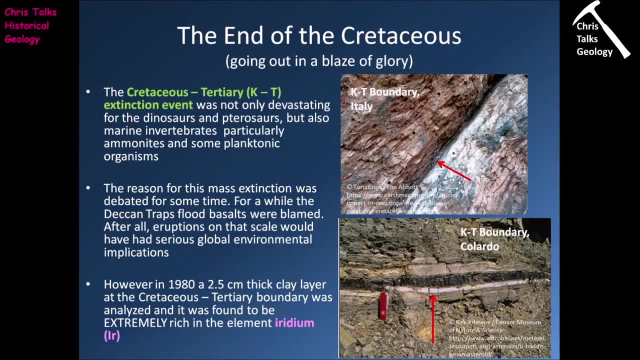 And that would obviously affect the ozone layer, and so that might lead to increased amounts of ultraviolet Radiation making it to the surface of the Earth. and so you can see how the Deccan Traps, you know, has the capacity at least to lead to a mass extinction, but it was never quite large enough. 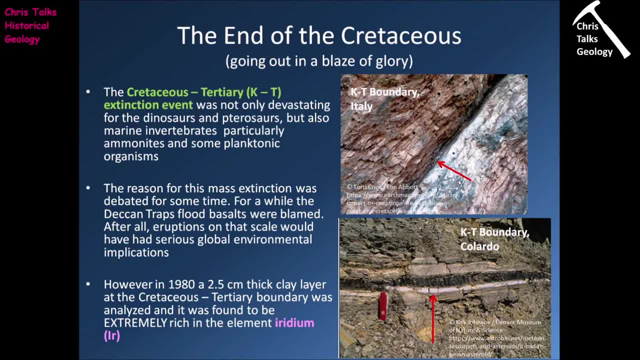 It was always a little bit difficult to explain how. you know, granted, a very large volcanic eruption was capable of causing a global and very, very powerful mass extinction event, So it didn't quite work. It was a good enough argument, but it just seemed a little bit slow. 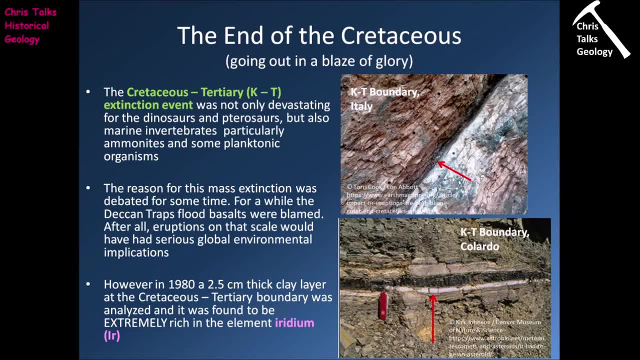 Small compared to the actual total size of the Cretaceous-Tertiary mass extinction. Now this changed in 1980.. So in 1980, a 2.5 centimetre thick clay layer at the Cretaceous-Tertiary boundary was analysed and it was found to be extremely rich in an element called iridium. 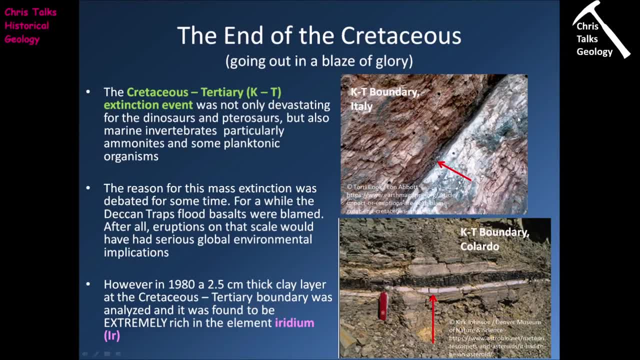 So just to give you some idea, this here is actually the layer of clay that was sampled, So you can see it's a clay layer that's running through here. There are limestones below it and limestones above it, And you can actually see there are some circles drilled into the rock here. 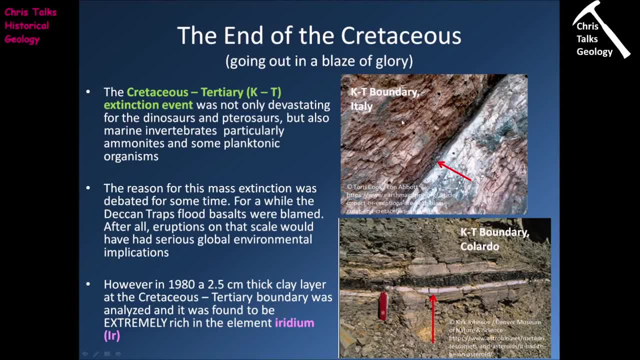 This is where rock samples have been taken for analysis, And so what some scientists were doing is they were just simply taking rock samples through this sequence and they were analysing them because they were trying to come up with a new dating method for dating sedimentary rocks. 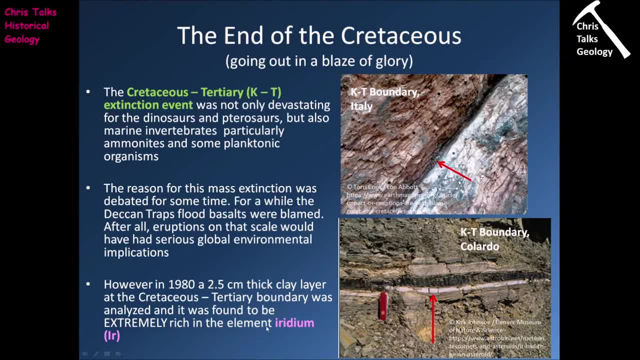 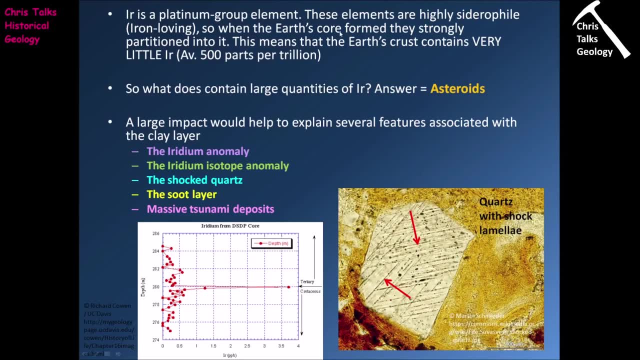 And it just so happened that one of the elements they were using to try and date the sedimentary rocks was iridium. Now, iridium is a very, very rich element. It's a very rare element. So because it's highly siderophile, that means iron-loving when the Earth went and formed its iron core. 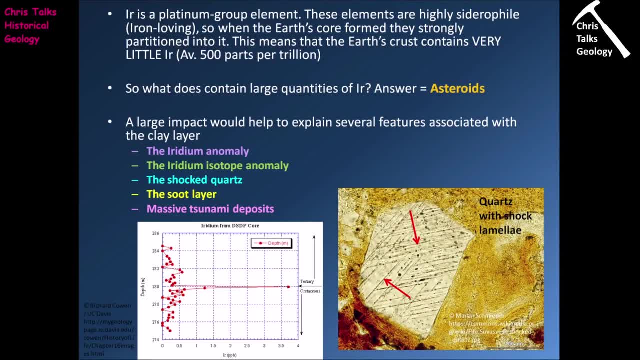 nearly all of the iridium that was present in the early Earth went and sequestered itself in the Earth's core, And so this means that the Earth's mantle and the Earth's crust is very, very iridium-poor. So, just to give you some idea, the average iridium concentration in the Earth's crust is 500 parts per trillion. 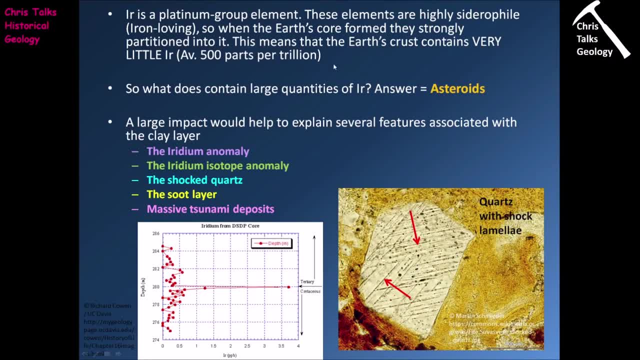 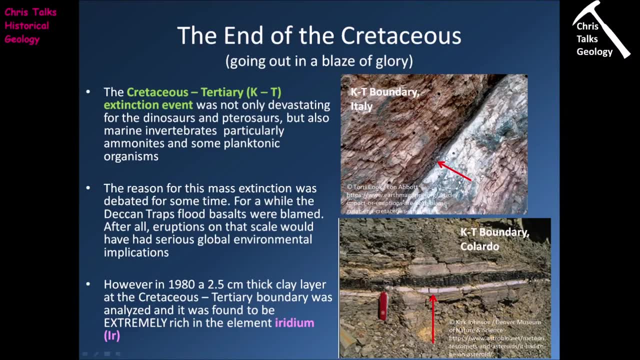 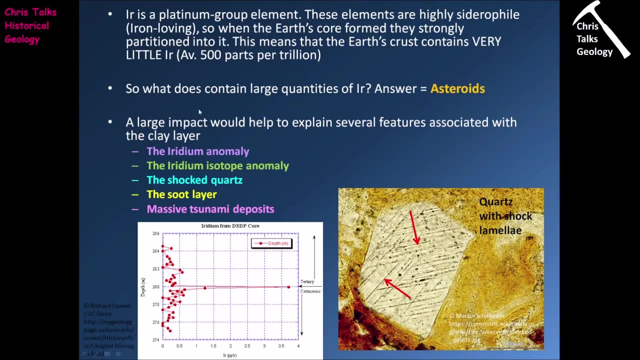 So that's a very, very low concentration. So the fact that we see this sudden increase in iridium in this clay layer here is extremely interesting to geologists. So the question then becomes is: right well, where do we find large quantities of iridium? 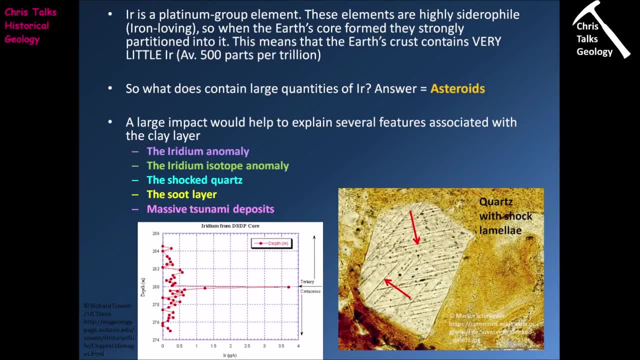 Well, you can find them in certain types of mineral deposit. However, this clay layer is absolutely nothing to do with the formation of ores, So iridium is a very, very low concentration. So the fact that we see this sudden increase in iridium in this clay layer here is extremely interesting to geologists. 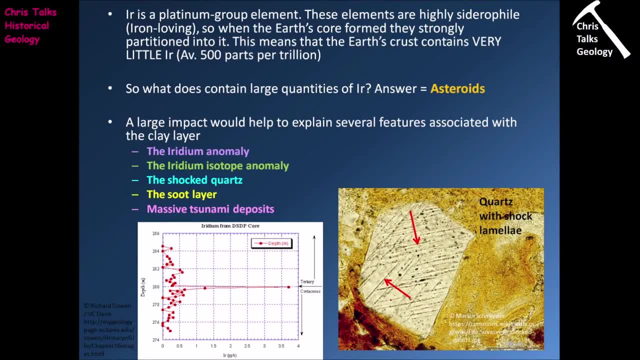 It's nothing to do with that process. The only other place where we find iridium in large concentrations is asteroids. So as soon as you see this iridium anomaly and as soon as you think, well, what could cause it, 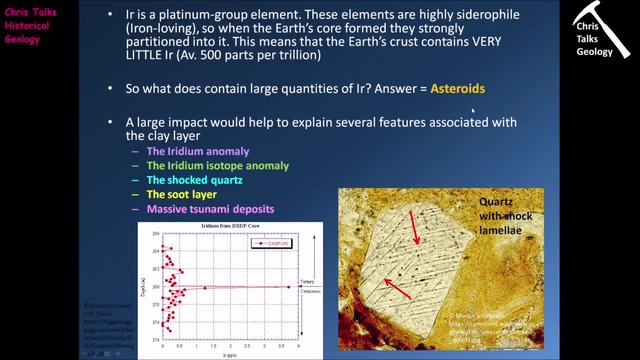 Well, asteroid is the only logical answer. Well then, all of a sudden, you begin to think: well, maybe the Cretaceous-Tertiary mass extinction is due to some kind of impact event. Now, once you have that idea, then you can go and look at the other evidence and you can see right. 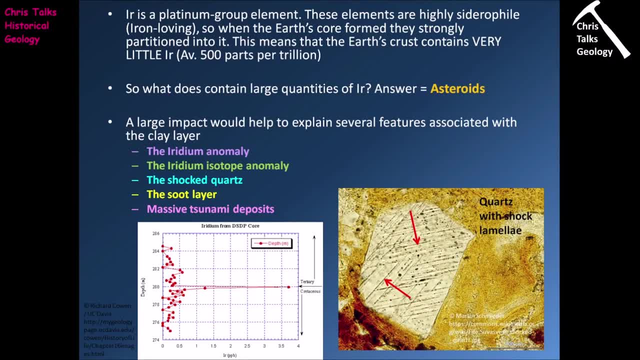 does an impact event matter? Does an impact event match with the evidence that I'm seeing? So obviously an impact event would be consistent with the iridium anomaly. The asteroid that would hit the Earth would have contained quite large quantities of iridium when compared to the concentration in the Earth's crust. 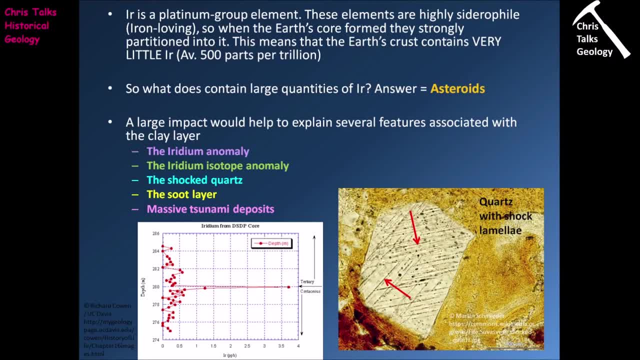 And so when the asteroid hit the surface of the Earth, obviously the asteroid would have been mostly destroyed. That would have thrown huge amounts of dust into the air and mixed in with that dust would have been pieces of the asteroid And that dust would essentially have fallen across the Earth. 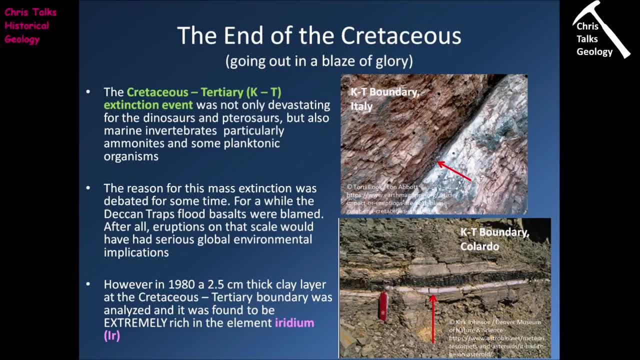 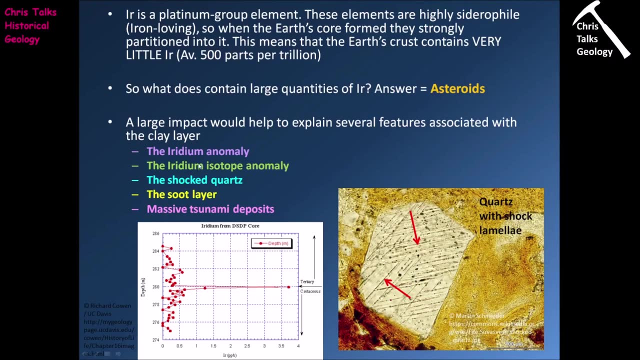 That dust would have fallen across the entire surface of the Earth and, essentially, this dust, this ejecta layer, would then go to form this clay horizon which we can see here and here. Another thing that we see is that we see that the iridium isotopes present in this clay layer are a little bit off. 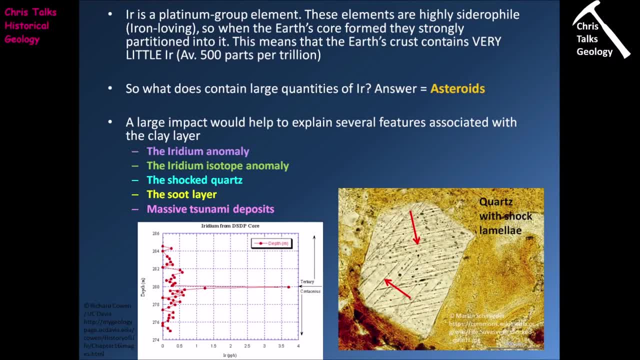 So the iridium isotope ratio that we see for the Earth is going to be different to the iridium isotope ratio that we get for things like air, And so when we look at the iridium isotopes present in this clay layer, we see that they are most closely related to the type of ratios which we would expect to find associated with asteroids. 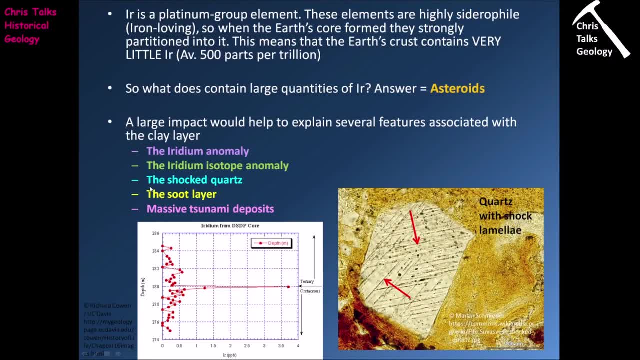 Now, another thing that we see is that we see in the rocks associated with the impact and as part of the clay layer, we have pieces of quartz which show a very, very distinctive texture, called shocked quartz. You can actually see a picture of it right here. 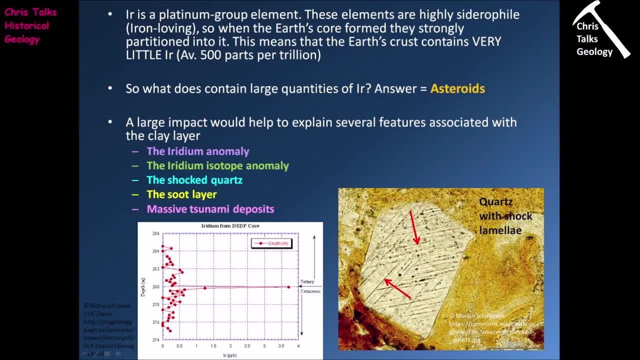 So here's a quartz crystal down a microscope, and you can see that it has all of these parallel lines. And these parallel lines are the result of, essentially, a pressure wave passing through the crystal, compressing it and deforming its internal structure. 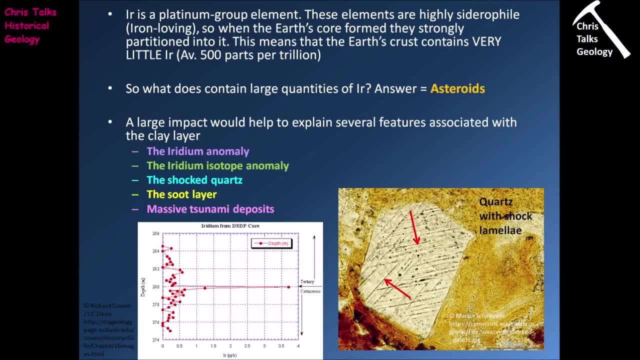 leading to the formation of these what are called shock lamellae within the crystal. Now, there are only two ways in which you get shocked quartz. The first one is a nuclear explosion And, to the best of my knowledge, the dinosaurs did not have nuclear weapons. 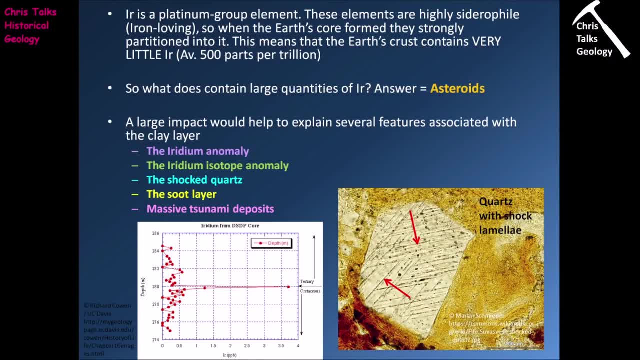 The other way that we can get shocked quartz is as part of a meteorite impact. And so you know, once again, meteorite impact is obviously going to produce an event which has very, very high pressures, very, very high temperatures, and this is going to lead to the formation of shocked quartz. 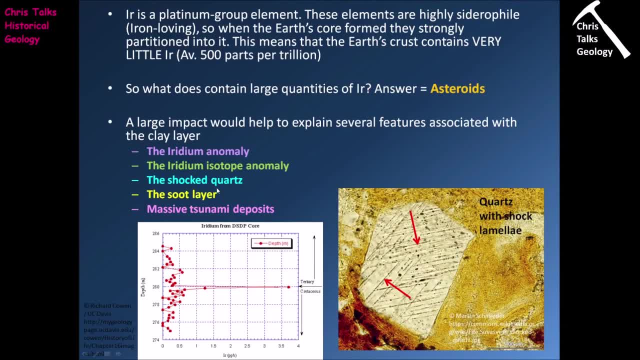 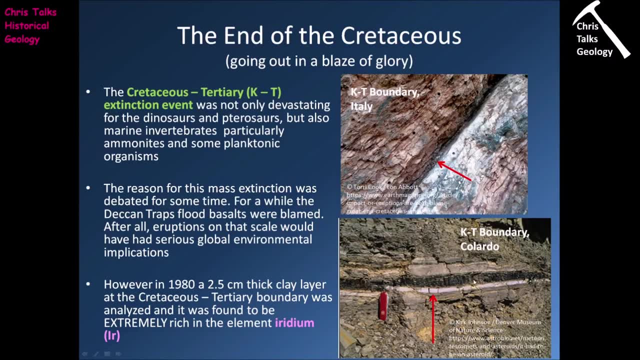 An impact would also go some way to explaining the soot layer. So if we just go back to the previous slide, you'll notice that above the clay layer right here you can see, you have this thick black, And this thick black band is full of organic material and it appears to be mostly made up of burnt plant material. 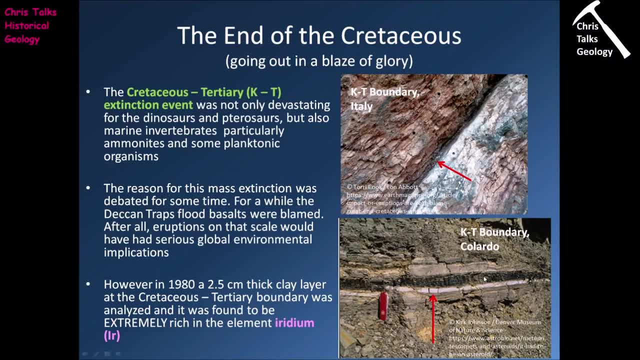 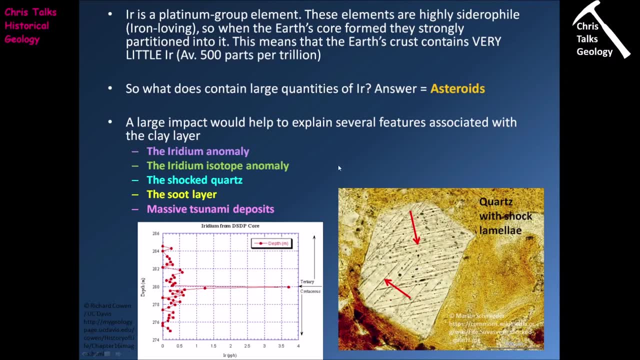 So the question is is: well, how did we end up with this big, thick layer of burnt material? And the chance is is that the material may well represent large scale forest fires associated with the impact event. Now, this point is argued over to some degree, so I'm just going to tell you that, for honesty's sake. 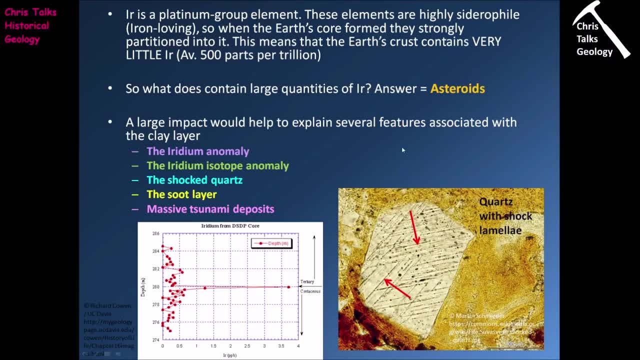 But the soot layer in theory could be tied in to an impact event. And the final thing that we see is, as part of the late Cretaceous sequence of rocks, in some areas we see the formation of massive tsunami deposits, So we see sedimentary rocks associated with tsunamis. 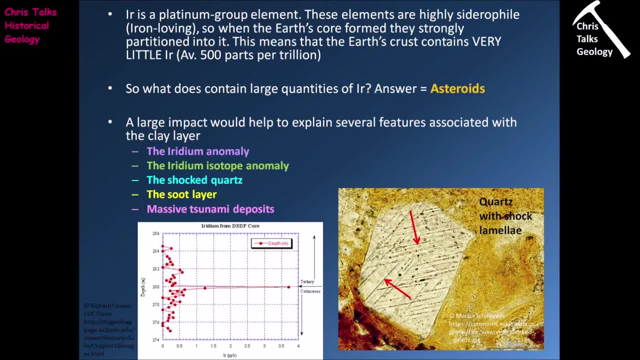 And the sedimentary rocks we're seeing for the end of the Cretaceous-Tertiary period. well, the Cretaceous-Tertiary boundary, should I say, show in some areas these huge, thick tsunami sequences which show there must have been a very, very large tsunami event. 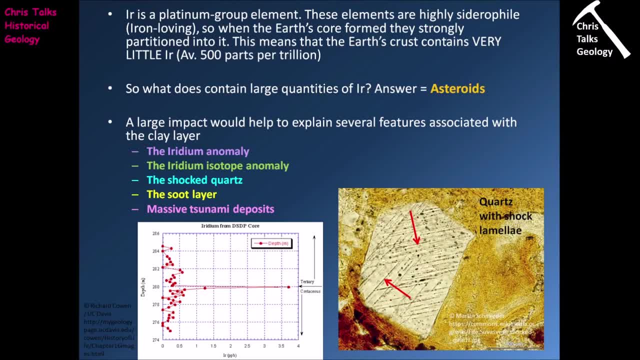 And once again, this would be consistent with an asteroid if the asteroid landed in the oceans or at least on the coast. So just to give you some idea about just how powerful, or just how big, should I say, this Iridium anomaly is. 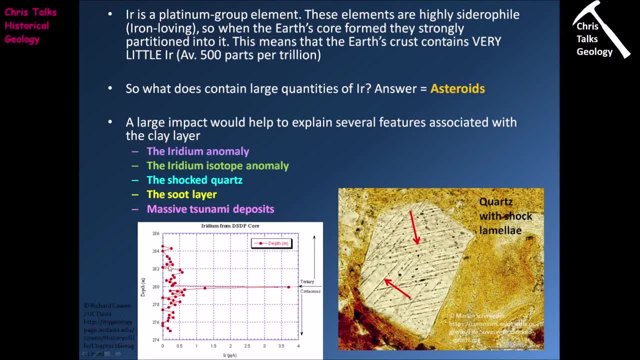 if we look at the graph here, you can see these are the standard ranges for Iridium within the Cretaceous-Tertiary boundary And you'll notice that in the limestones below and above the clay layer and you'll notice that as you hit the clay layer. 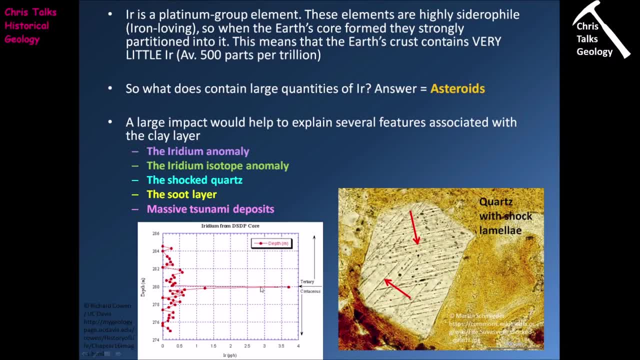 which marks the Cretaceous-Tertiary boundary, you have this huge spike in Iridium concentrations. So you're going from about half a part per billion Iridium over here to over three and a half parts per billion Iridium over here. 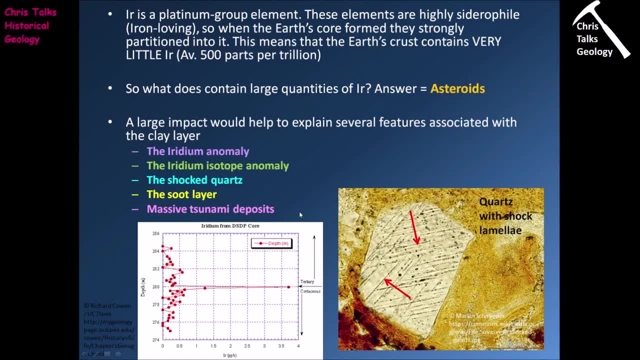 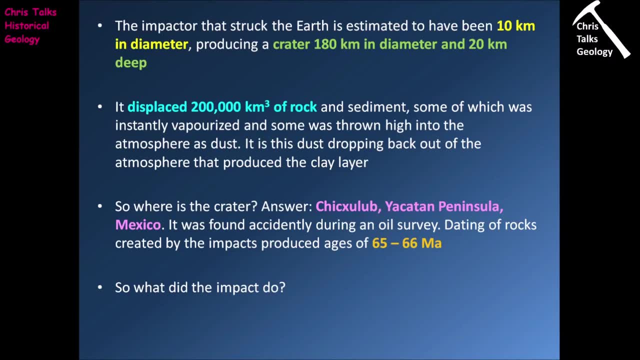 That's quite a substantial increase. So once you realize that an asteroid is the most likely cause of the Cretaceous-Tertiary mass extinction, you can begin to, you know, think about. well, how big would the asteroid have had to have been? 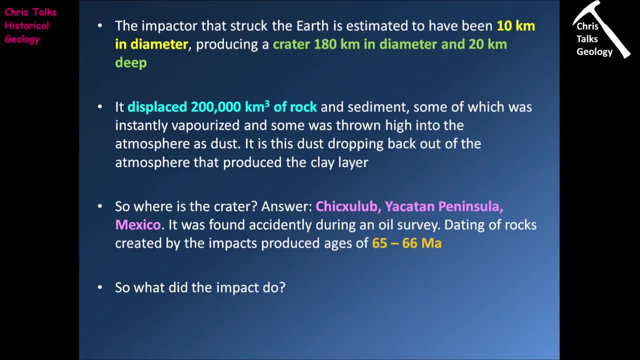 to cause the level of destruction that we see, And our calculations suggest that the asteroid in question would have probably been about 10 kilometers in diameter and it would have produced a crater that was 180 kilometers in diameter and about 20 kilometers deep. 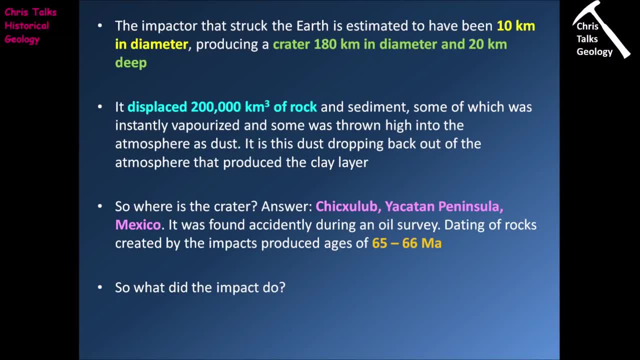 So this is obviously a very big hole in the ground. Now, the formation of this crater will have displaced about 200,000 cubic kilometers of rock and sediment, And a lot of this rock and sediment would either have been instantly vaporized by the impact or it would have been turned into very, very fine dust. 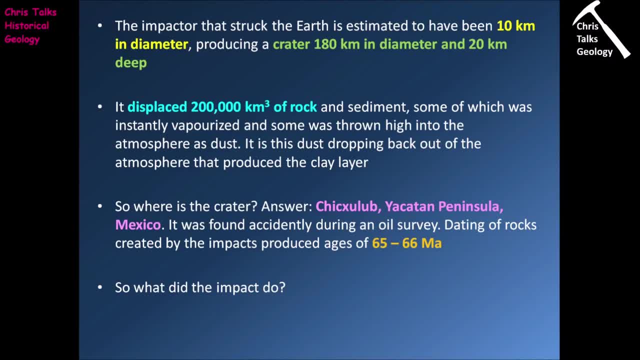 that would have been thrown up into the atmosphere. This fine dust is referred to as ejecta because it's getting ejected from the impact crater. So this dust would have gone up into the atmosphere and it would have done a couple of things. Number one, the dust would have blocked out the sun. 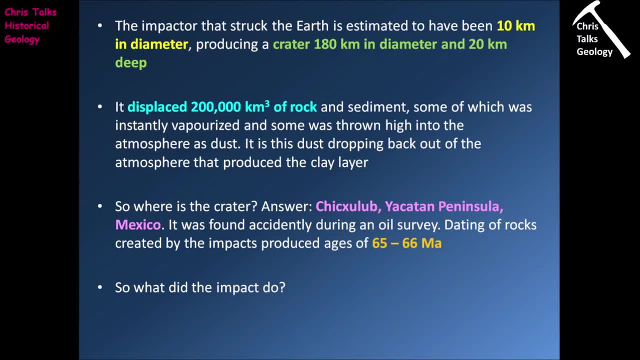 because the dust in the air is going to stop sunlight making it to the surface of the earth. This is obviously going to have an effect on photosynthesizing organisms and, of course, it's going to lead to their eventual demise. So the other thing that we see is that, as the dust falls out of the atmosphere, 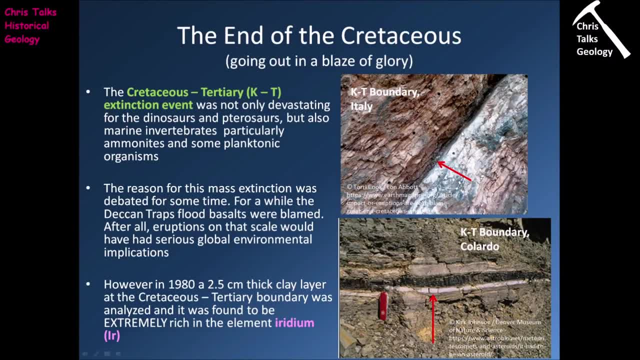 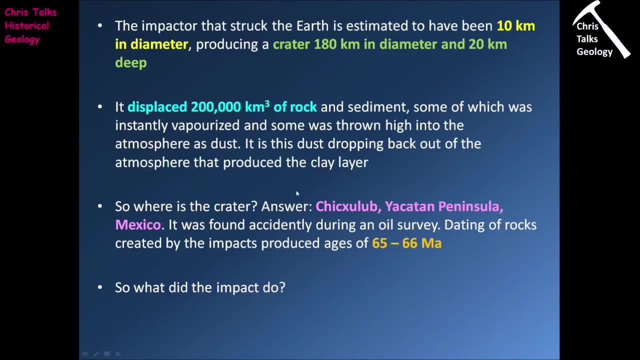 it's going to lead to the formation of an ejecta layer, which we see as the clay horizon, this clay layer right here. So the next question is: well, where is the impact crater? And we're very, very lucky in that we managed to find the impact crater. 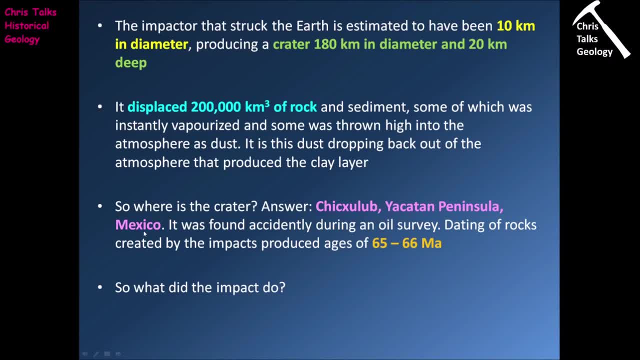 It's located on Chicxulub, which is part of the Yucatan Peninsula of Mexico. Now, the crater itself was actually found accidentally during an oil survey. But once they had found it, they started taking samples and they identified the crater and they managed to date it to 65 to 66 million years ago. 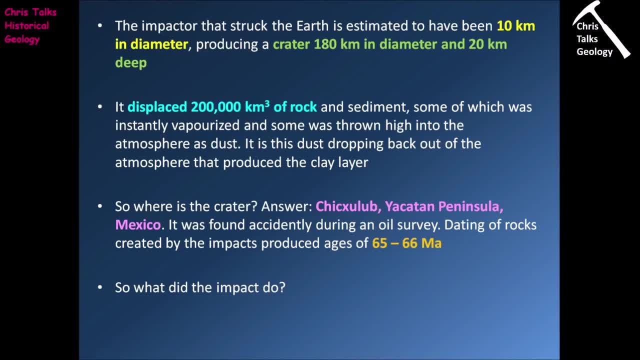 which is again a very, very long time ago. So the impact crater is located on Chicxulub, which is part of the Yucatan Peninsula of Mexico, And it's located exactly on the Cretaceous-Tertiary boundary, exactly when this mass extinction occurred. 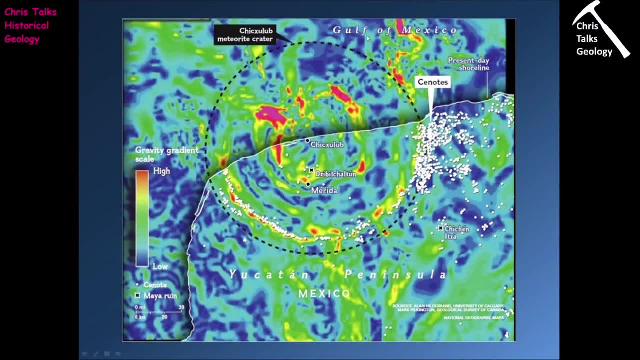 So what did the impact actually do? Well, if we look here, we can see this is a gravity map for the Yucatan Peninsula. So here we have the coastline of Mexico running along here, So to the south we actually have dry land. 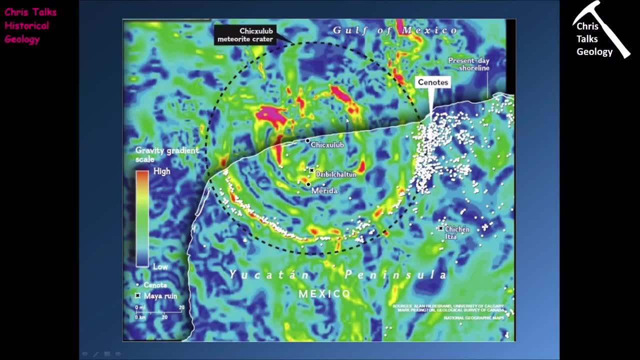 and to the north we have the Gulf of Mexico And what you can see is, if you look at the gravity map, you can see you have these circular features associated there and you have a semicircular feature that's coming around here. 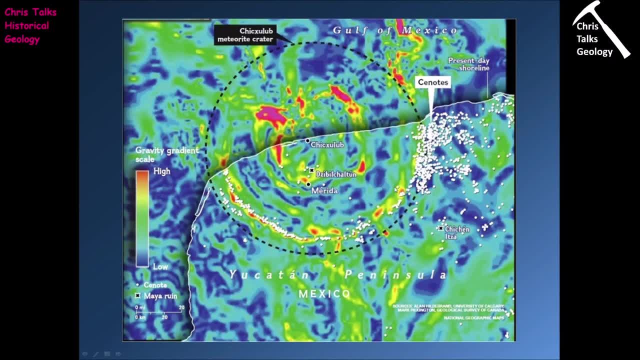 And these are the faults which are associated with the formation of the crater. So these are the results of the crater forming process, And so by looking at these, we can actually work out where the edge of the crater will fall. Now, another thing that we see is because the rocks in the area got very, very heavily faulted. 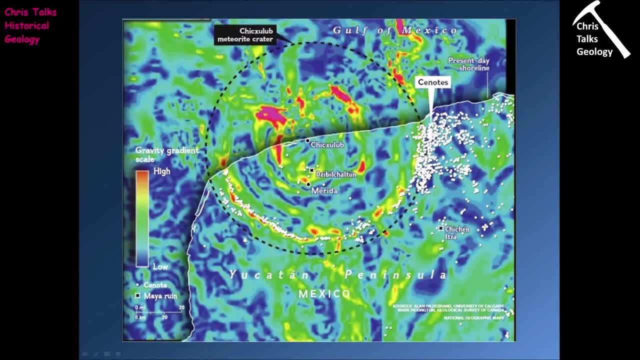 as part of the crater making process. it means that these faults in the ground are going to be, are going to be exploited by water, So you're going to get water moving underground using the fault planes as a path of least resistance, And so, because the rocks in this area are mostly made of limestones. 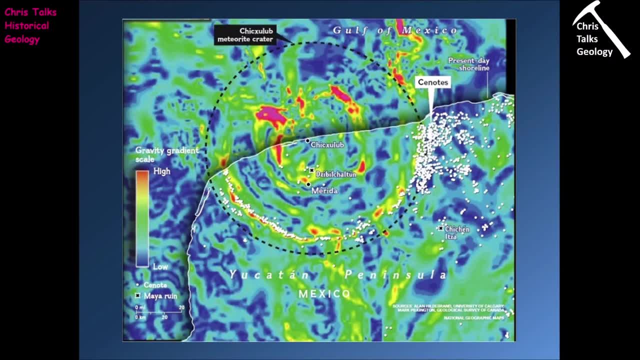 the passage of the water along these fault planes is going to lead to the formation of caves And eventually the roofs of these caves will fall in and this is going to lead to the formation of sinkholes. And so if you look here, we have all of these white spots on the diagram. 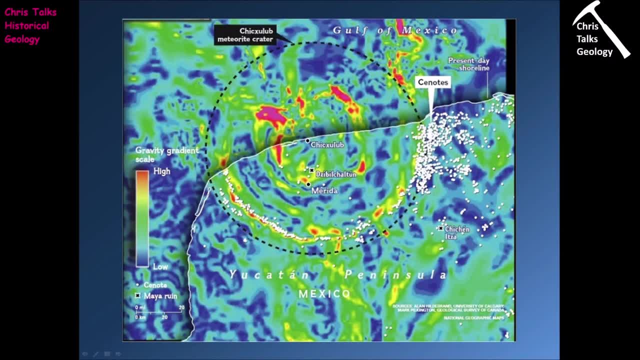 and these are the holes that are going to form the sinkholes. And so if you look here, we have all of these white spots on the diagram and these are all sinkholes, And what you'll notice is there's a distinct band of sinkholes coming around here. 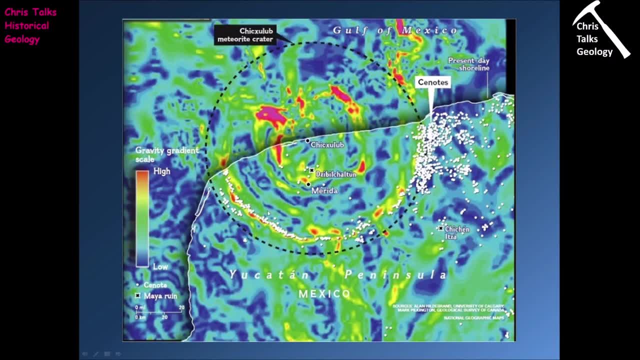 which is associated with this gravity high, And so what you're seeing here is you're seeing, essentially, sinkholes forming along one of these very, very large faults, which was part of the crater forming process, And so this is another piece of evidence that shows us that we have a crater here. 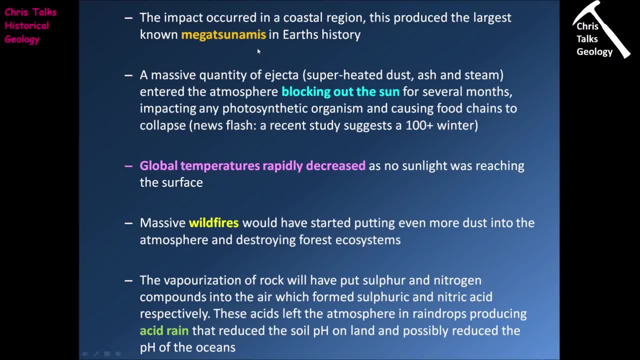 So we know the impact will have occurred in a coastal region And this obviously helps to explain the presence of the mega-tsunami deposits because, of course, if the meteorite goes into the oceans, of course that's obviously going to lead to the formation of a very, very large tsunami. 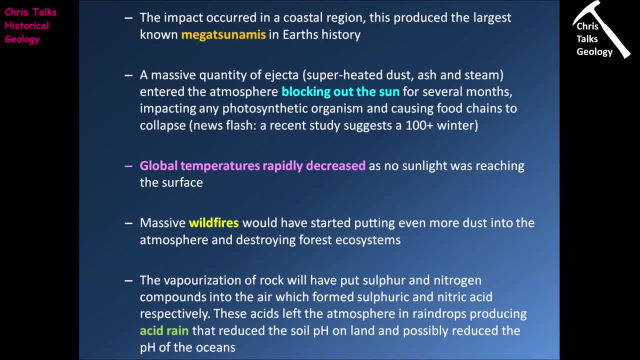 Now the ejector, the material that's thrown out during the impact event, is obviously going to enter the atmosphere, and a lot of that material is going to end up blocking out the sun. Now, this period of time could have lasted anywhere from several months to a more recent study. 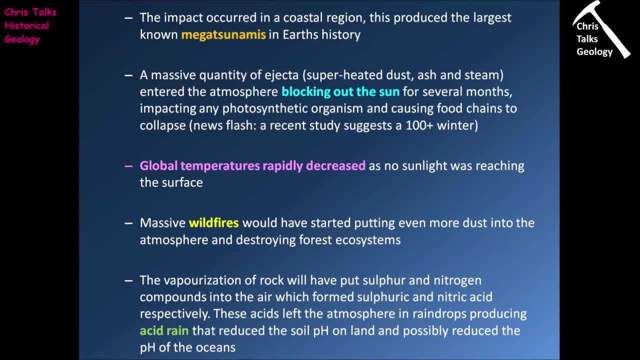 which suggests the sun could have been partially blocked out for anywhere in excess of 100 years. So this is, you know, an interesting problem. We know that the sunlight would have been blocked out by all this dust in the atmosphere. One of our issues is how long it took for that dust to exit the atmosphere and for sunlight. 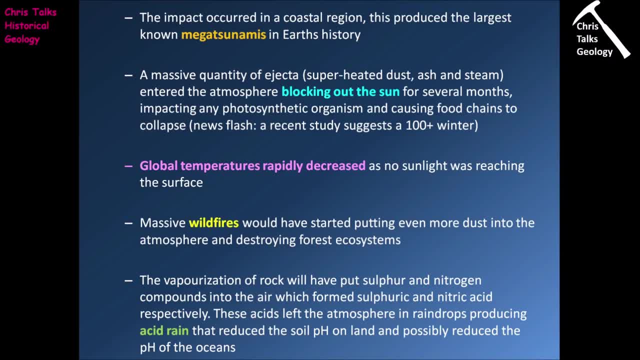 to make it back onto the surface of the earth in reasonable quantities. So the loss of this sunlight obviously would have been detrimental for photosynthesizing organisms and so obviously we will have seen a lot of those photosynthesizing organisms dying off. 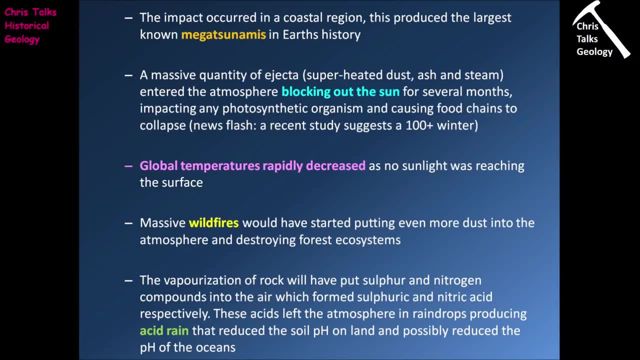 Of course, this is going to then cause the food chain to collapse, because these small photosynthesizing organisms are essentially at the base of the food chain in the marine environment. Obviously, because we're blocking out the sun, we're also going to see a decrease. 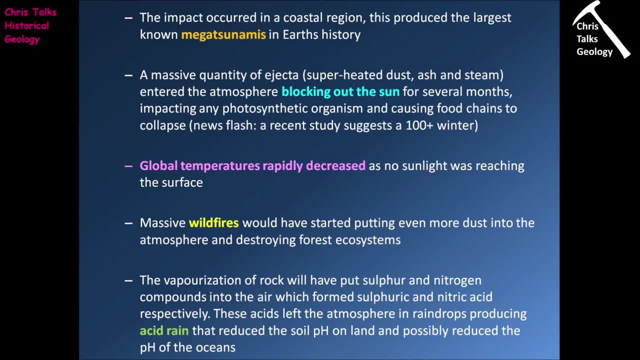 in global temperatures because no sunlight is making it to the surface of the earth, So that means far less solar radiation. Obviously, as we've discussed, we're going to see the onset of massive wildfires associated with the impact, and this is going to lead. 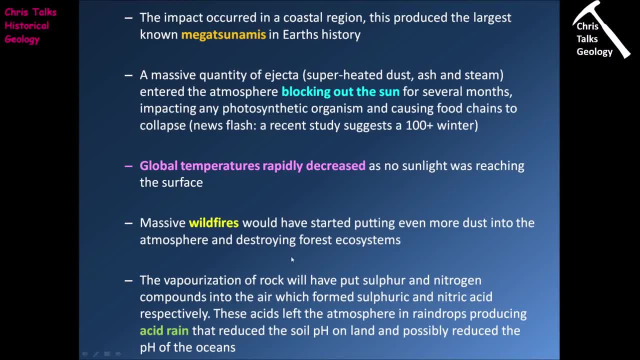 to the destruction of large areas of forest. It's also going to lead to large amounts of carbon dioxide being put into the atmosphere. The other thing that we notice is that the rock which is vaporized by the impact ended up putting quite large quantities of sulfur and nitrogen into the air. 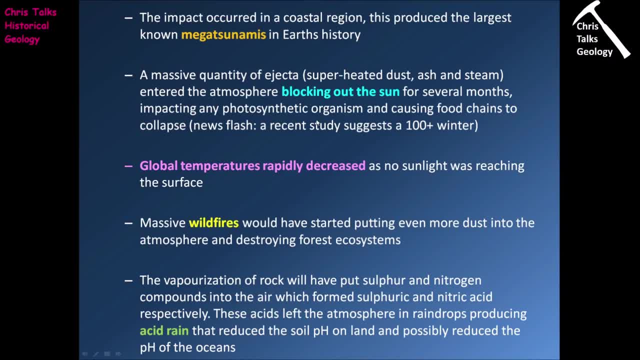 So it just so happens that the marine sediments tend to be relatively rich in sulfur, And so this means that when these marine sediments were vaporized as part of the impact event, a lot of that sulfur went into the atmosphere. And, of course, when you have sulfur and you mix it with water, 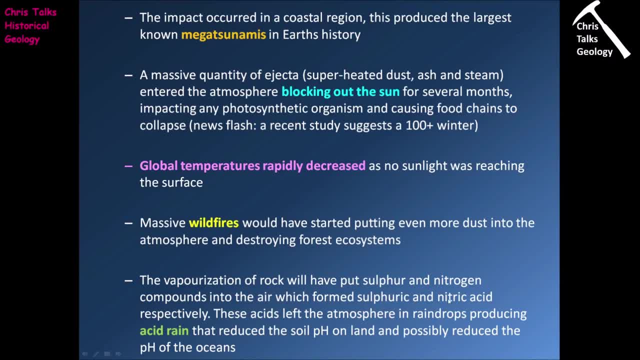 you end up forming sulfuric acid. When you have nitrogen, you mix it with water. you can end up forming nitric acid, And so this is going to lead to acid rain. And, of course, acid rain is very, very bad because, depending on where it lands, 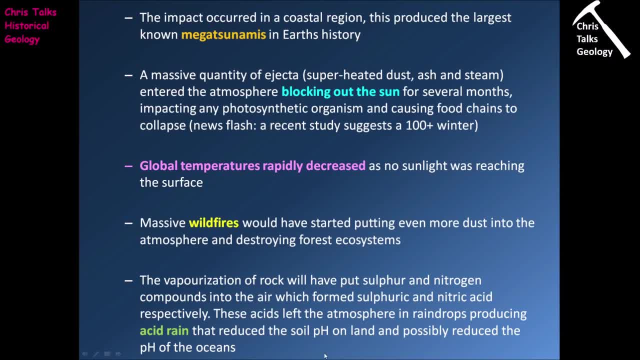 it can either cause the pH of soil to decrease or it could even, in extreme cases, cause the pH of the oceans to decrease, And of course, this is going to be very, very bad. If soil pH decreases, so it becomes more acidic, that can kill the roots of plants. 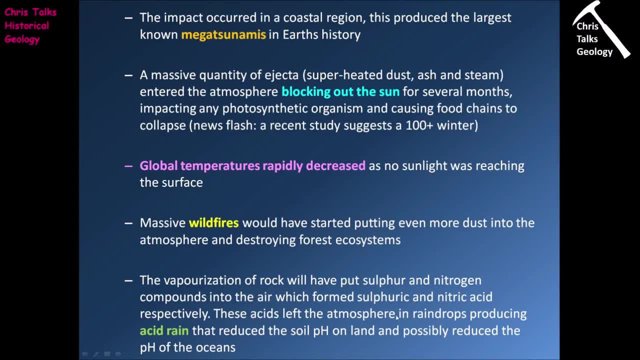 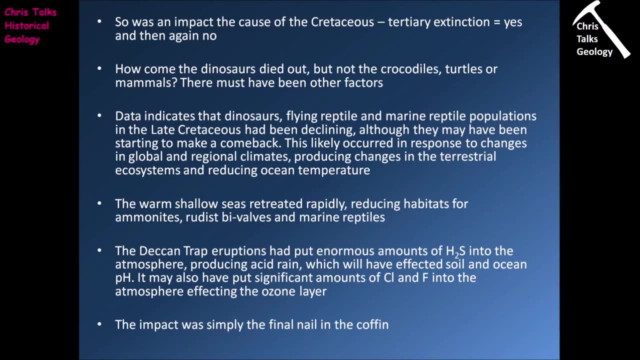 And if the pH in the oceans decreases, that can make it very difficult for animals that have carbonate shells to survive, because the carbonate is going to be constantly reacting with the more acidic water. So was an impact the cause of the Cretaceous-Tertiary extinction. 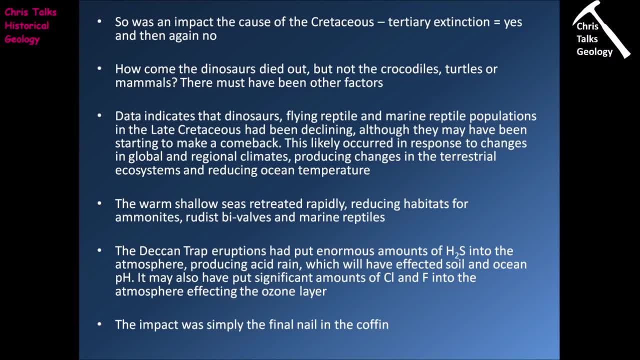 The answer is yes and then again no. So one of the questions we have to ask ourselves is: how come the dinosaurs died out, but the crocodiles, the turtles and the mammals managed to make it through? There clearly have to have been other factors. 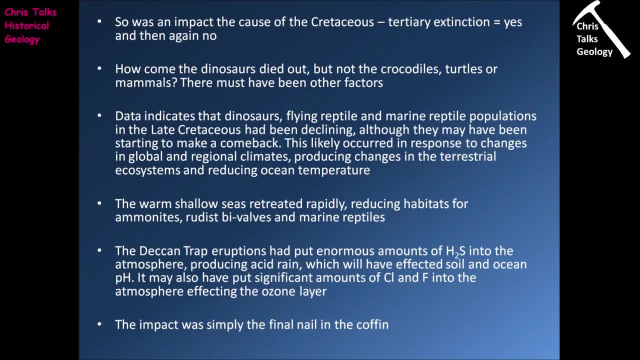 There have to have been other factors operating during this time period. Now data indicates that the dinosaurs, the flying reptiles and marine reptile populations in the late Cretaceous had, on the whole, been declining, And so this would suggest that the dinosaurs were already in trouble. 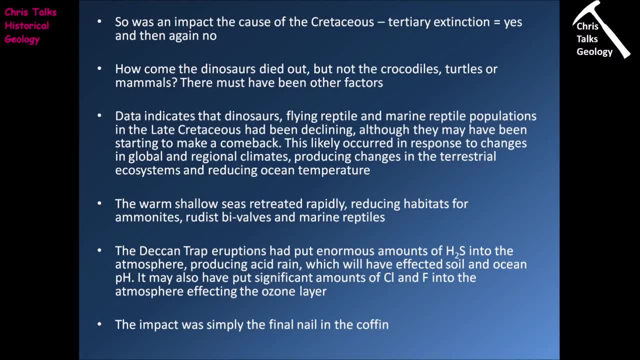 There is, however, some evidence to suggest that right at the end of the Cretaceous, the dinosaurs might actually have been making a bit of a comeback, But it looks like this Cretaceous-Tertiary mass extinction seems to have been a bit of a comeback. 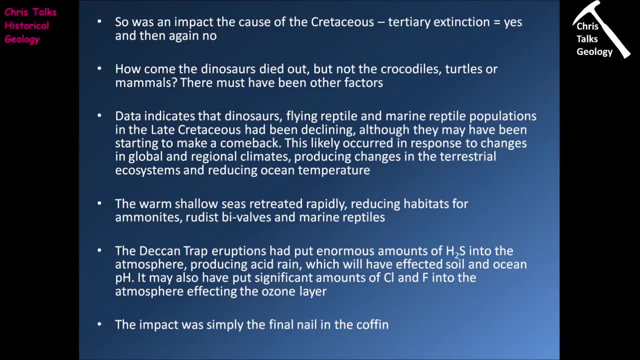 So we're going to put a stop to that. So the change in the dinosaur populations that we see as we're moving through the Cretaceous is likely a response to the change in global and regional climates which are being produced as the continents move towards their current positions. 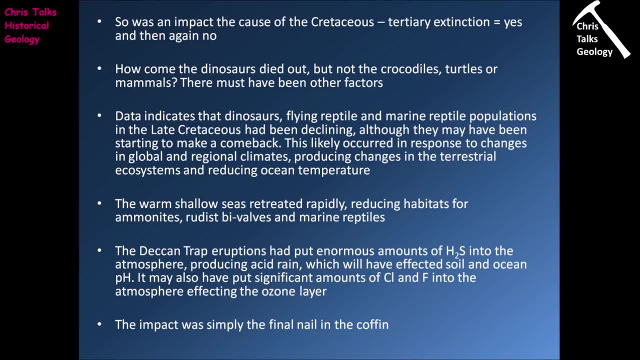 At the same time, we're obviously going to see a change in ocean currents as well, as the continents move towards their current positions, And so that's going to affect marine organisms, And so what we see is we have both populations of animals on the land and in the oceans. 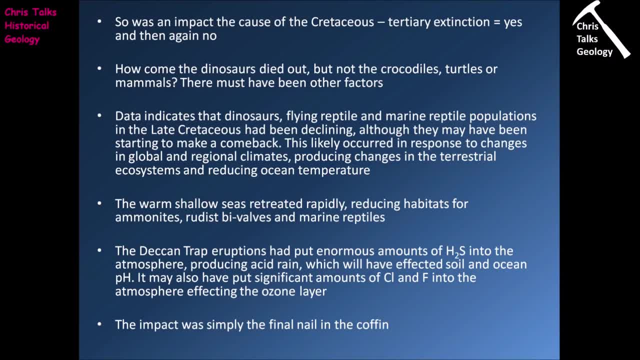 which are already being stressed by the breakup of Pangea and the movement of the continents towards their current locations, And then, on top of that, we then obviously have this impact. So, in terms of marine environments, we see that the warm shallow seas 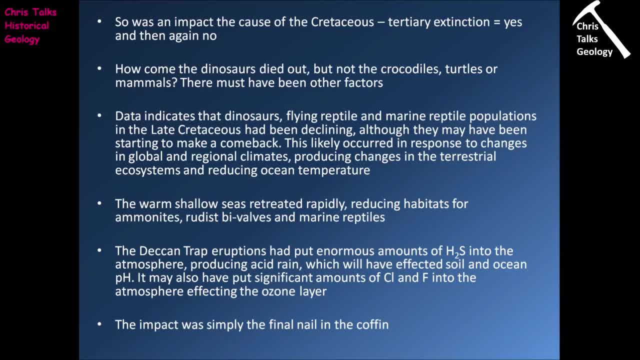 which we had throughout much of the Mesozoic, especially in the Cretaceous, are also rapidly regressing, And so this is going to mean that habitats for animals like ammonites, rudest bivalves and marine reptiles 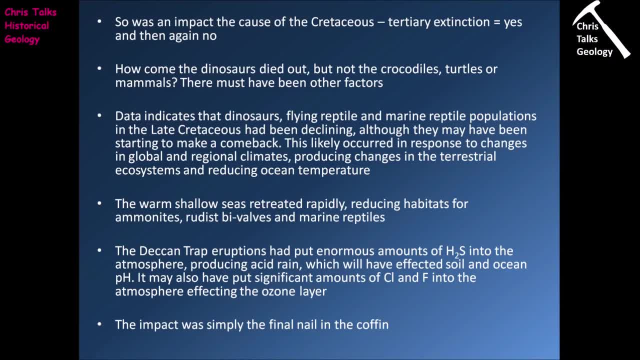 essentially are going to be reduced, And so obviously that's going to make it more difficult for them to survive. We also still have the Deccan Traps eruption going on in India. That's going to be putting out huge quantities of sulfur dioxide into the atmosphere. 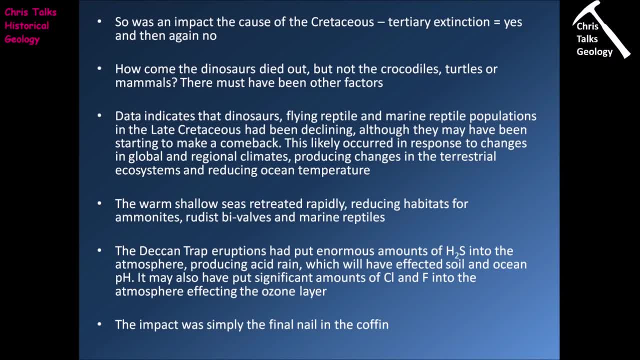 that's going to react with water to produce sulfuric acid. That's going to lead to acid rain And we're also going to have the eruption putting out large quantities of chlorine and fluorine, and that's also going to go into the atmosphere where it's going to react with ozone. 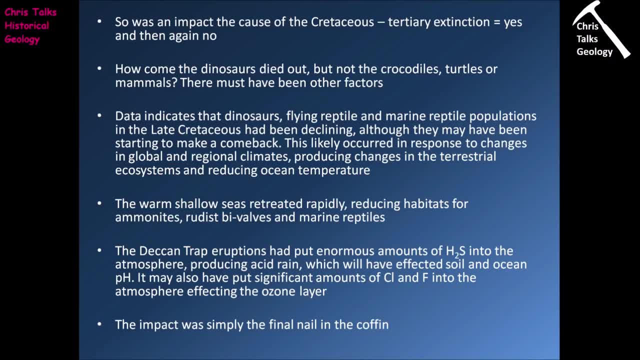 So it's going to degrade the ozone layer. So what you essentially have is you have a situation where the dinosaurs, the flying reptiles, the marine reptiles, the ammonites, the rudests and other marine organisms are already in a pretty bad situation. 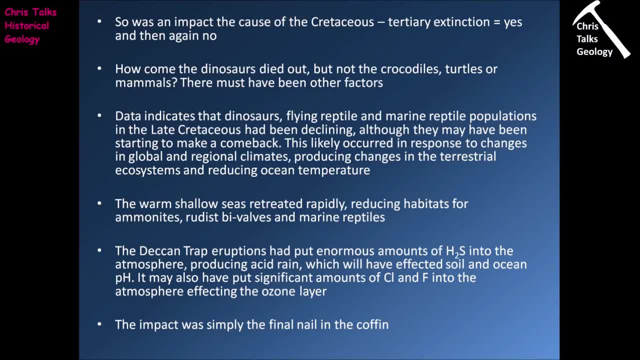 And then, just to top it off, you get this huge impact occurring, and that pretty much finishes them off. In contrast, other groups of animals like the crocodiles, the turtles and the mammals were, on the whole, doing pretty well in the Cretaceous. 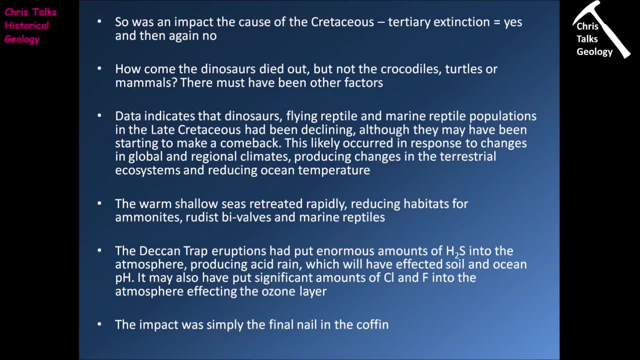 So it looks like they were on a relatively firm footing before this impact occurred, and so that managed to help them to make it through this event and make it into the Cenozoic, where they could then start diversifying. Okay, everybody, so that's it for this lecture.